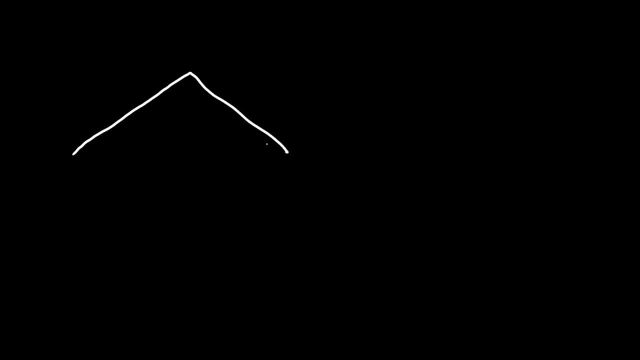 In this video we're going to focus on the rhombus. So what do you know about a rhombus? What are some features of a rhombus? A rhombus is a special type of quadrilateral. It's a four-sided polygon. 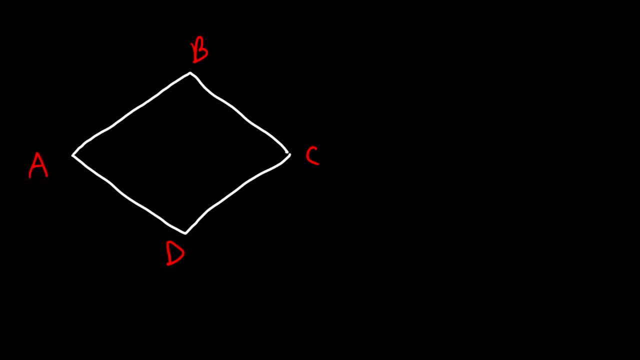 and it's also a parallelogram. So AB is parallel to DC. So we can write that like this: Opposite sides are parallel, And so we could say that DA is parallel to CB. Now for a rhombus, like a square. all sides are congruent, They all equal each other. 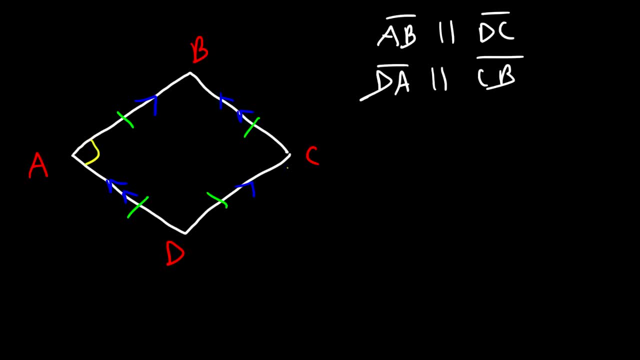 Opposite angles are also congruent. So angle A and angle C are congruent, And so we can say that DA is parallel to CB. They have the same measure, And also angle B and angle D have the same measure as well. So let's say, if angle A is 80 degrees, angle C will be 80 degrees as well. 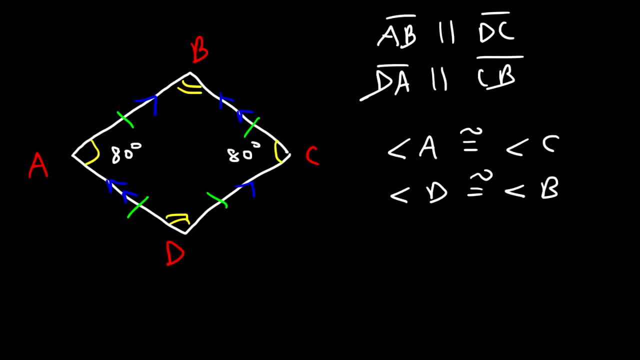 Now, consecutive angles are supplementary Because these lines are parallel. these lines, these angles are same side interior angles Or consecutive interior angles. Any add up to 180.. So angle A plus angle B is 180.. So this is 100 and this is 100. 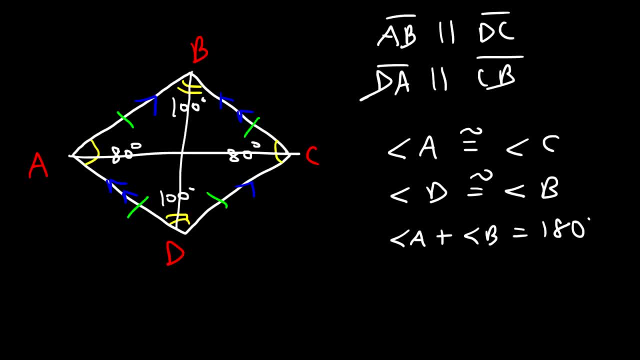 Now let's say, if we draw two diagonal lines, what's gonna happen? Now, you need to know that the diagonals, they bisect the angles. So let's use the same thing figure and let's draw the diagonals here. so this was a hundred. now this is going. 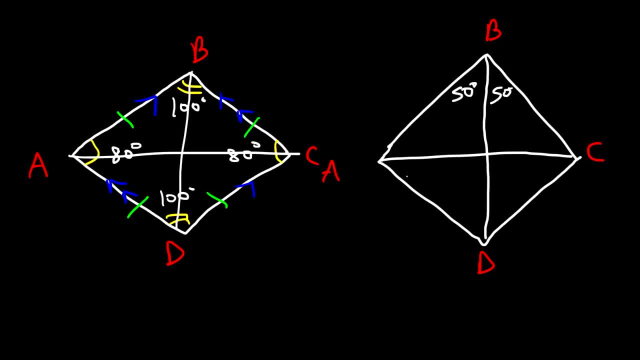 to be 50 and 50, and this was 80. so this is split up into 40 and 40, and this two over here is 50 and 50. now the three angles of a triangle must add to 180. so therefore, what is this angle here? it's. 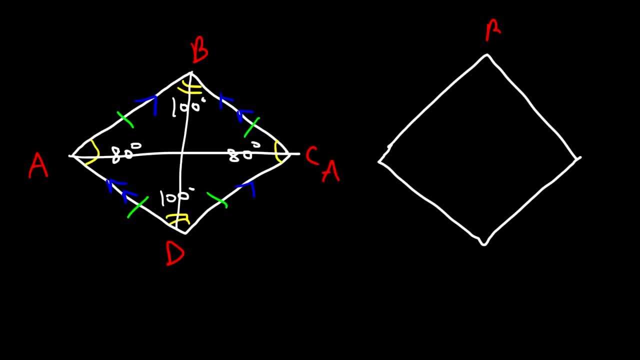 So let's use the same formula, Same figure and let's draw the diagonals here. So this was 100, so now this is going to be 50 and 50.. And this was 80, so this is split up into 40 and 40. 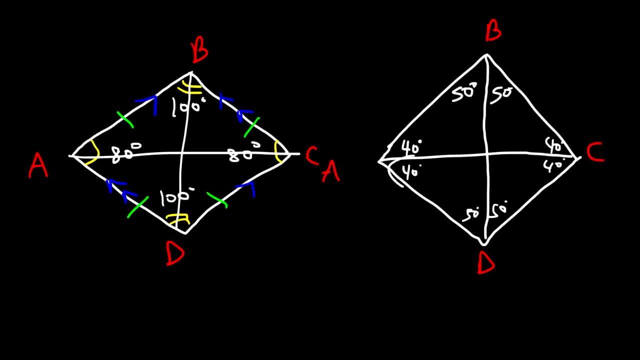 And this two over here is 50 and 50. Now the three angles of a triangle must add to 180.. So, therefore, what is this angle here? It's 180 minus 40 minus 50. And this comes out to be 90.. 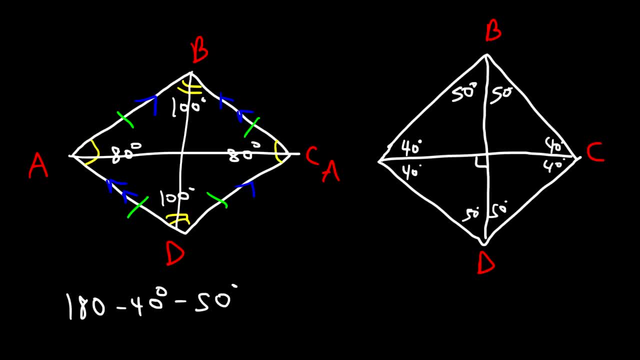 So what this means is that the diagonals, they bisect each other. They're perpendicular bisectors, they bisect each other at right angles. So let's call this E. It turns out that AE, AE, AE is congruent to EC and BE is congruent to ED. 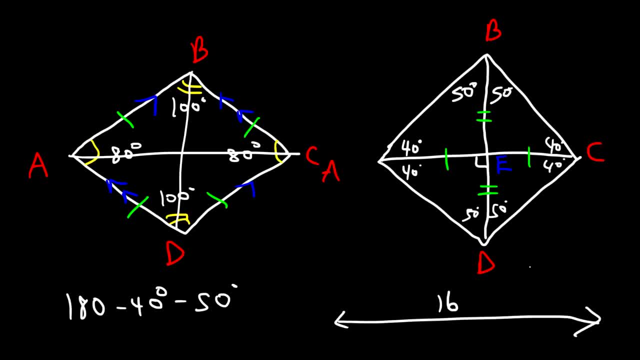 So let's say if AC was 16 units, AE would be half of that and EC would be half of that as well, So they would both be 8.. Now let's say if BD was 20 units, BE will be 10, and ED is 10 as well. 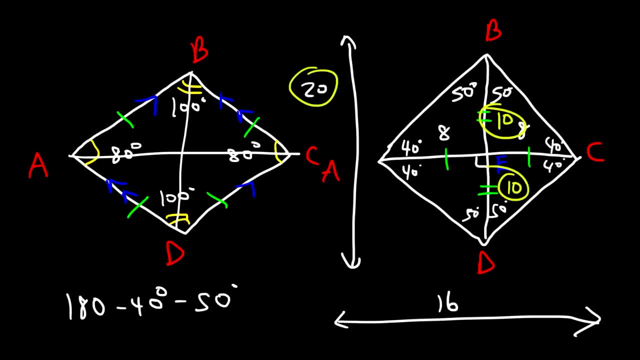 So these two would add up to 20.. And they have to be equal to each other. Now the area of a rhombus is 1 half D1 times D2. So this 20 could be D1, and this 16 could be the second diagonal D2.. 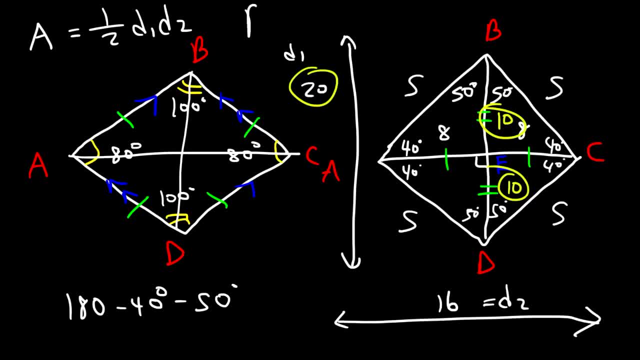 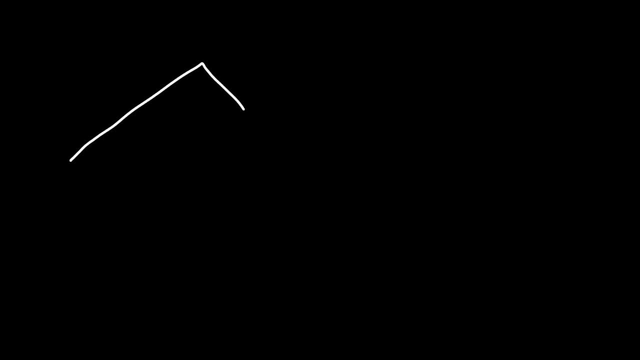 And all of the sides are congruent, So the perimeter is simply going to be 4S. Now let's work on some example problems. So let's say: if we have this rhombus ABCD, And let's say that AC is equal to 8.. 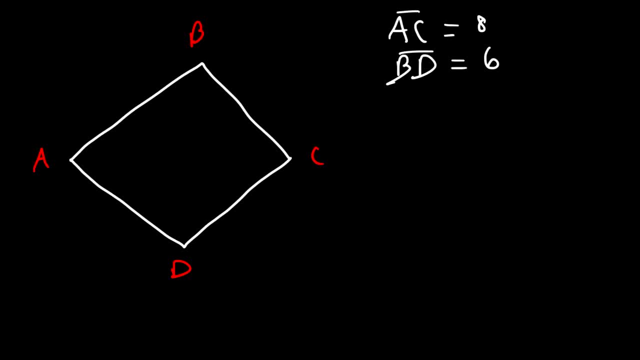 And BD is equal to 6.. Calculate the area of the rhombus and at the same time determine the perimeter. So feel free to pause the video. So AC is the first diagonal, Which is 8. And BD is the second diagonal. 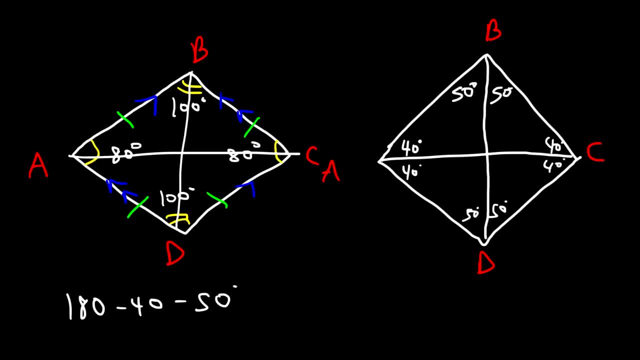 180 minus 40 minus 50, and this comes out to be 90. so what this means is that the diagonals, they bisect each other, their perpendicular bisectors, they bisect each other at right angles. so let's call this e. it turns out that a e. 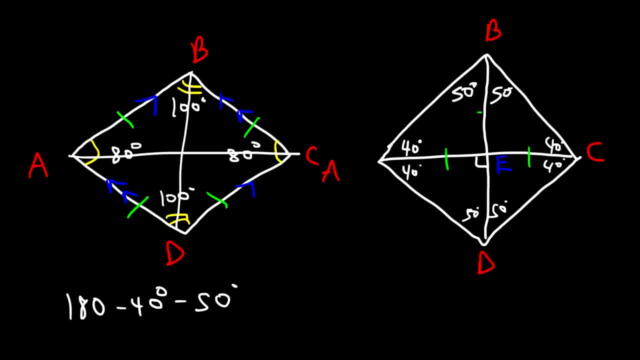 is congruent to ec and be is congruent to ed. so let's say, if a- C was 16 units, a e would be half of that and ec would be half of that as well, so they would both be 8. now let's say, if BD was 20 units, be. 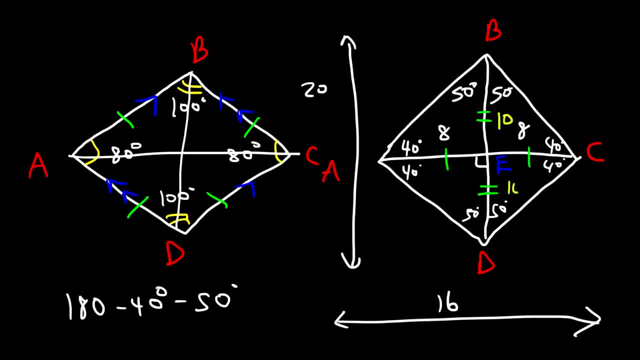 e will be 10 and ed is 10 as well, so these two would add up to 20 and they have to be equal to each other. now the area of a rhombus is 1 half d1 times d2, so this 20 could be d1 and the 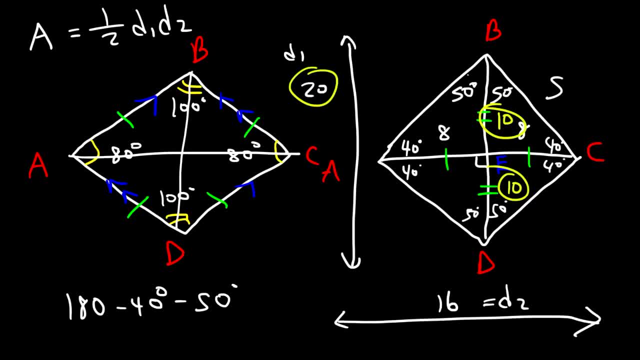 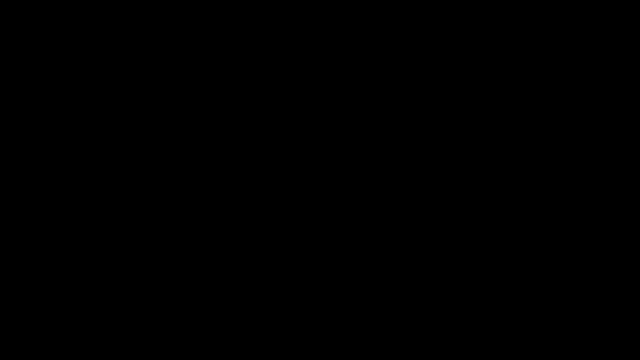 16 could be the second diagonal, d2, and all of the sides are congruent, so the perimeter is simply going to be 4s. now let's work on some example problems. so let's say, if we have this rhombus, ABCD, and let's say that AC is equal to 8 and 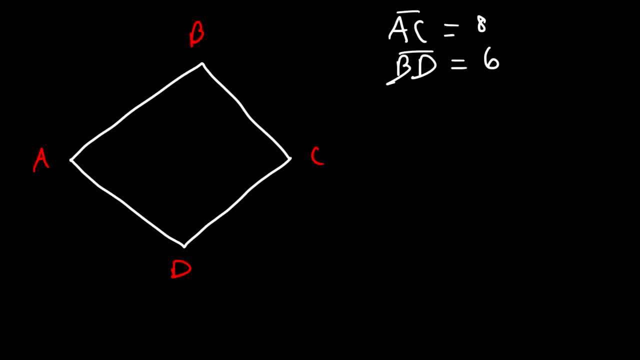 BD is equal to 6. calculate the area of the rhombus and at the same time determine the perimeter. so feel free to pause the video. so AC is the first diagonal, which is 8, and BD is the second diagonal. let's see if I can put it here and so 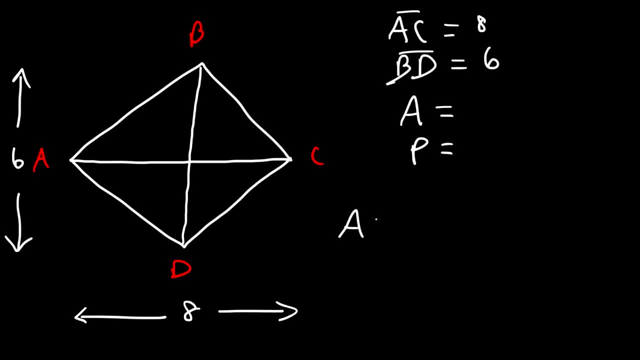 that's 6. so the area is 1 half d1 times d2. so d1 is doesn't matter which one's d1. we could say d1 is 6 and d2 is 8. half of 6 is 3. 3 times a is 24. so the 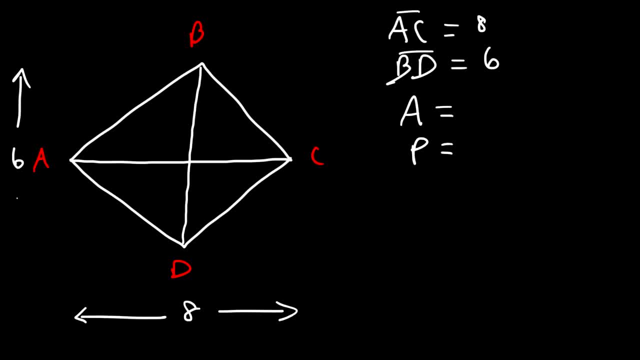 Let's see if I can put it here. And so that's 6.. So the area is 1 half D1 times D2. So D1 is doesn't matter which one is D1, we can say D1 is 6, and D2 is 8.. 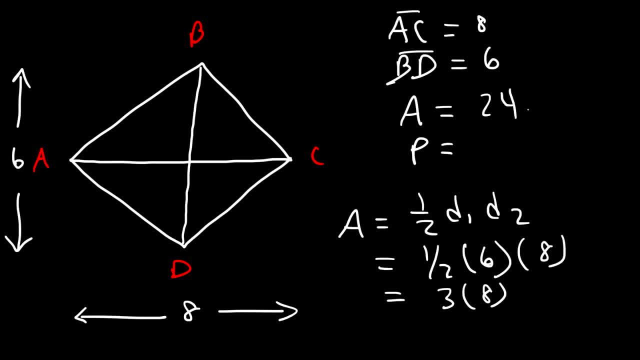 Half of 6 is 3, 3 times 8 is 24.. So the area of this particular rhombus Is 24 square units. Now how can we calculate the perimeter? Well, we need to calculate the side length S. 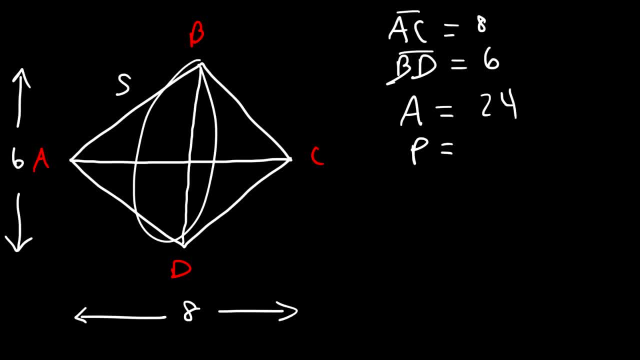 So if BD is 6. Then BE- let's say E is the. this point here- BE has to be 3. And ED has to be 3. And if AC is 8. That means AE has to be half of that, 4.. 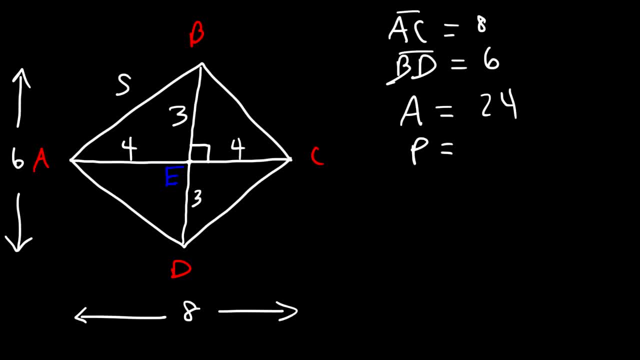 And EC is 4.. And also we have a right triangle. So now let's focus on this right triangle. here We need to calculate the hypotenuse, which we'll call S. So S squared is equal to A squared plus B squared. 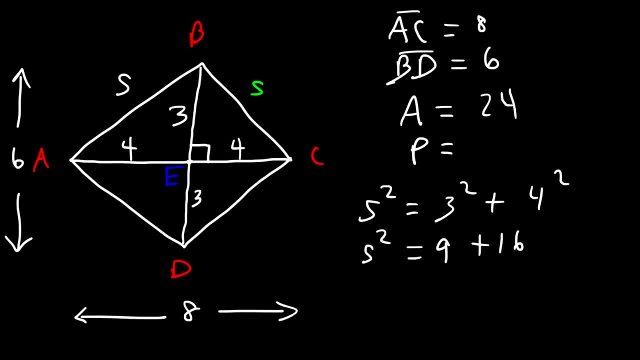 Three squared is 9.. Four squared is 16.. Nine plus 16 is 25.. So now we're going to take the square root of both sides. So the side length is 5.. Now we know the perimeter is 4S. 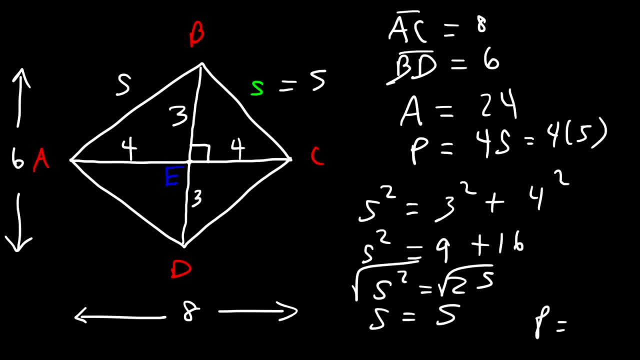 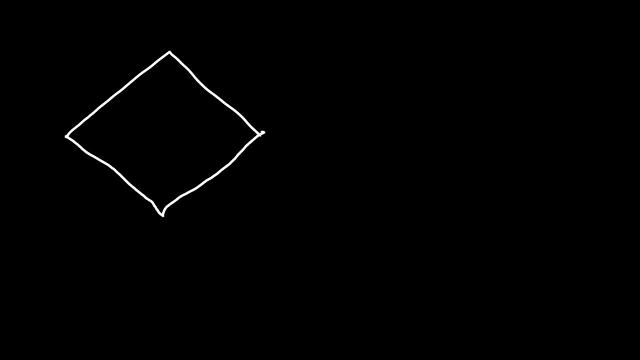 So that's 4 times 5.. And so the perimeter in this example is 20.. It's 20 units long. So that's how you can calculate the area and a perimeter of a rhombus. So here's the third question. 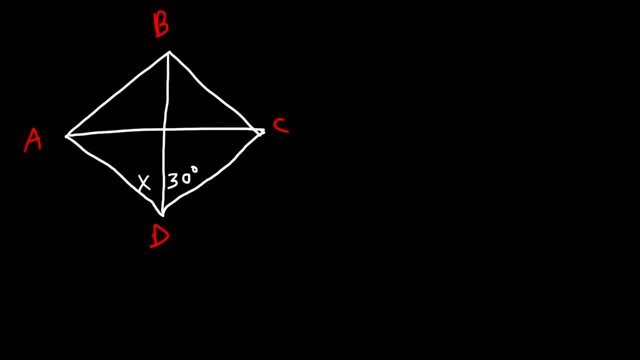 So let's say this is X, Yes, and this is 30 degrees. Let's say this is Y and this is Z. Determine the values of X, Y and Z. So now, the first thing we need to keep in mind is that. 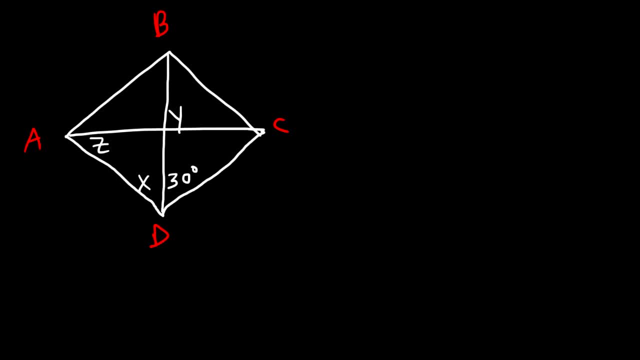 the diagonals bisect each other at 90 degrees, So this is the right angle, this is 90, and this is 90. So notice that these two are vertical angles, so they're congruent. Therefore, Y has to be 90.. 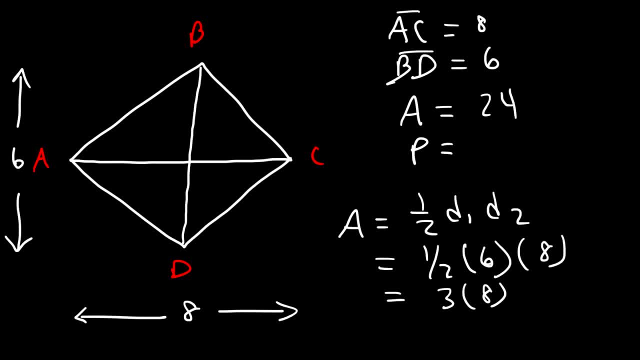 area of this particular rhombus is 24 square units. now, how can we calculate the perimeter? well, we need to calculate the side length s. so if BD is 6, then be e- let's say e is the. this point here- be e has to be 3 and ed has to be 3. and if 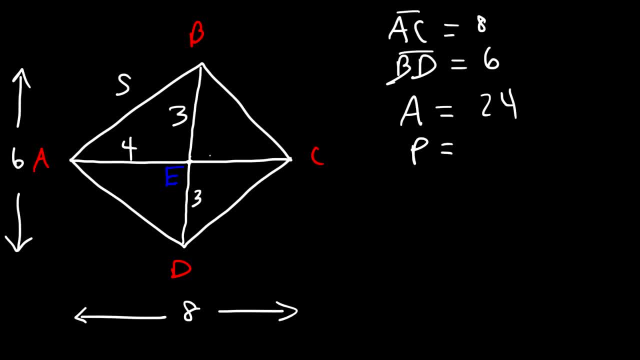 AC is 8. that means a e has to be half of that 4, and EC is 4, and also we have a right triangle. so now let's focus on this right triangle. here we need to calculate the hypotenuse which will call s, so s. 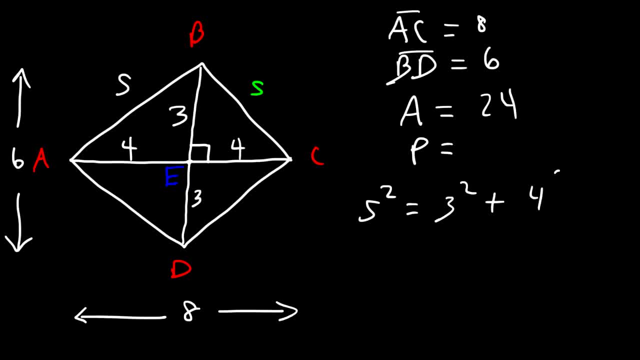 squared is equal to a squared plus b squared. 3 squared is 9, 4 squared is 16. 9 plus 16 is 25. so now we're going to take the square root of both sides. so the side left is 5. now we know the. 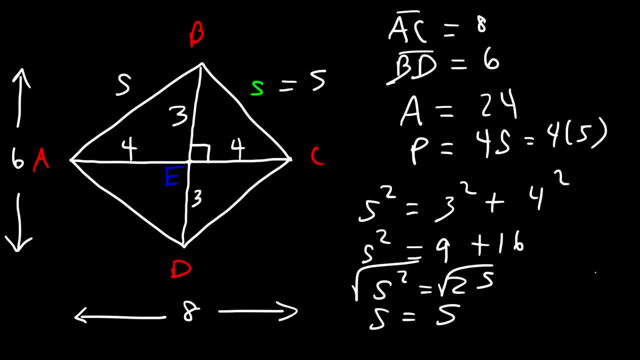 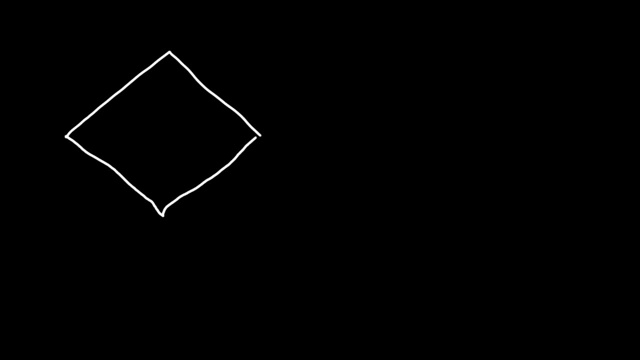 perimeter is 4s, so that's 4 times 5, and so the perimeter in this example is 20. it's 20 units long. so that's how you can calculate the area and the perimeter of a rhombus. so here's the third question. 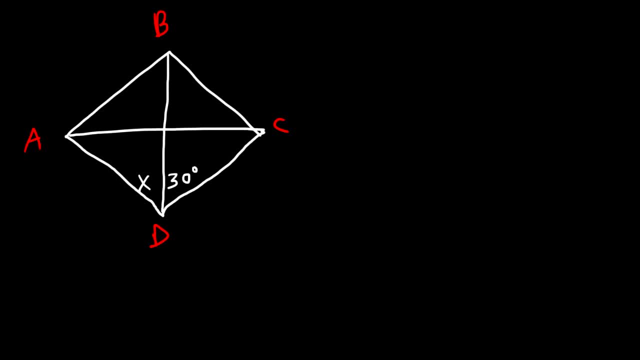 so let's say this is X and this is 30 degrees. let's say this is Y and this is Z. determine the values of X, Y and Z. so now, the first thing we need to keep in mind is that the diagonals bisect each other at 90 degrees. so this is the 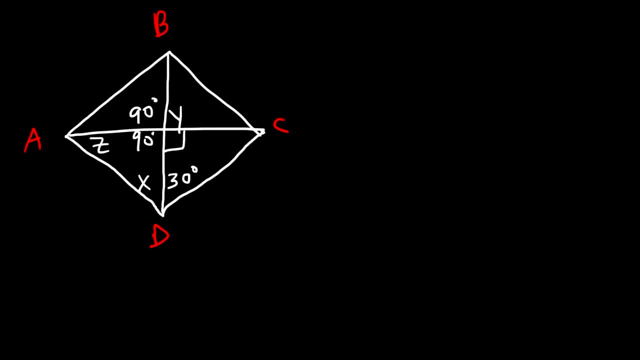 right angle. this is 90 and this is 90, so notice that these two are vertical angles, so they're congruent. therefore, Y has to be 90. now, the next thing that we need to keep in mind is that the diagonal will bisect this angle into two congruent angles, so 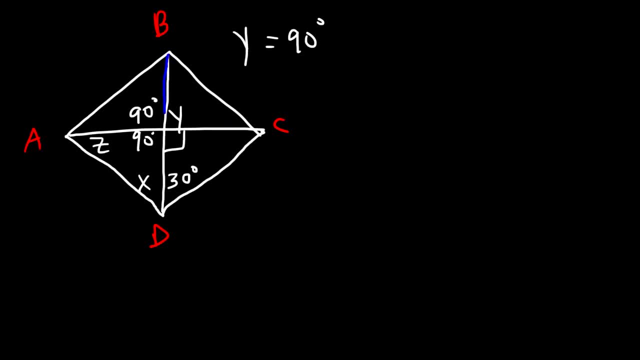 Now the next thing that we need to keep in mind is that the diagonal will bisect this angle into two congruent angles, So angle ADB has to be congruent to angle CDB. So if these two are equal to each other, that means X. 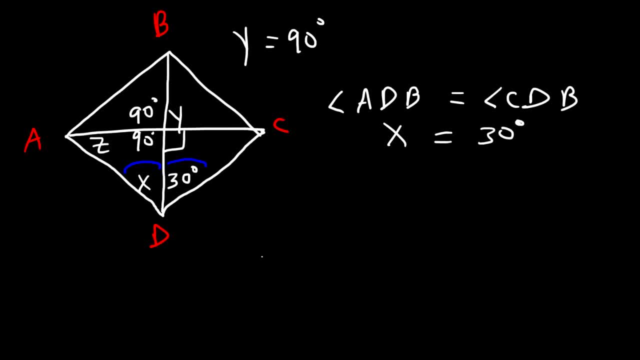 has to equal 30.. Now we can calculate Z. So if we focus on this triangle, we can see that this is 90, this is Z and this is 30. So Z plus 30 plus 90, the three interior angles of a triangle must add up to 180. 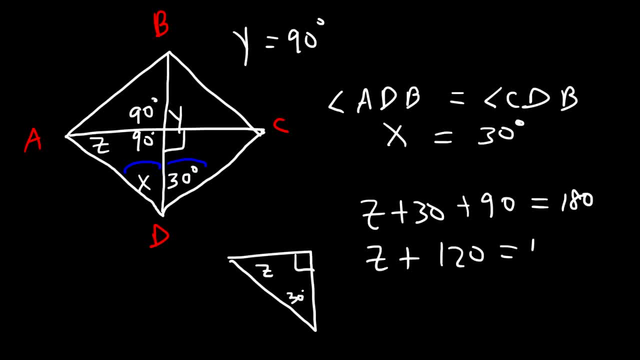 30 plus 90 is 120, and 180 minus 120 is 60. So these two angles, they're complementary to each other. they have to add up to 90 and these three combined, or they have to add up to 180. so that's how you could calculate the. 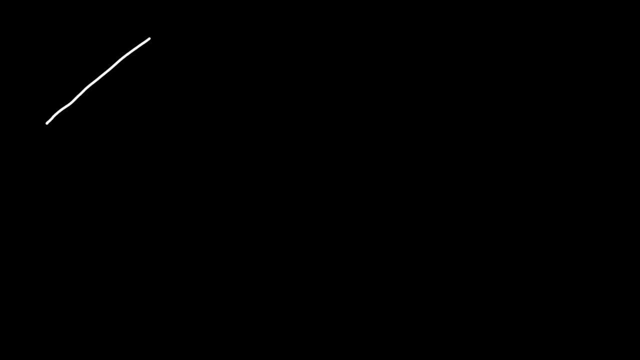 missing angles of a rhombus. so here's the next example problem that you can work on. so once again we have rhombus ABCD and this is going to be E. so let's say that AE is equal to 3x plus 1 and EC is equal to 5x minus 9. so with this, 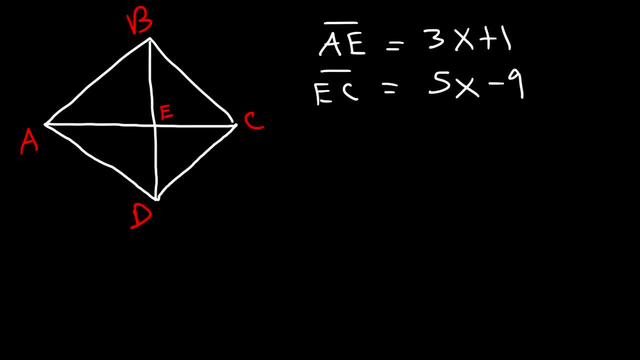 information, and let's say that also AB is 20, so this information calculate the value of BE. so go ahead and pause the video. try this problem. so we know that AE and EC are congruent because each diagonal bisects the other one, the perpendicular bisectors of each other, which makes E the midpoint of AC. so 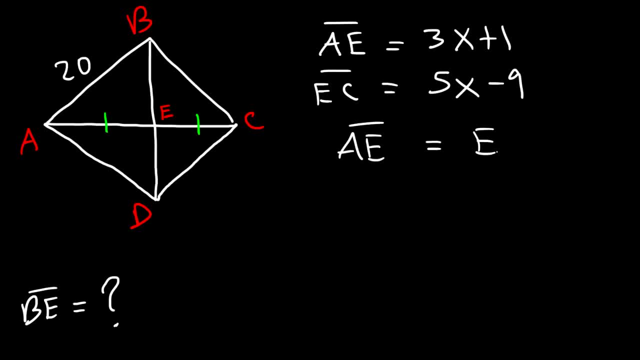 therefore we can say that AE and EC are equal to each other, which means that 3x plus 1 is equal to 5x minus 9. so let's subtract both sides by 3x and let's add 9 to both sides, so 9 plus 1 is 10, and 5x minus 3x is 2x. now let's divide both sides by 2, so 10. 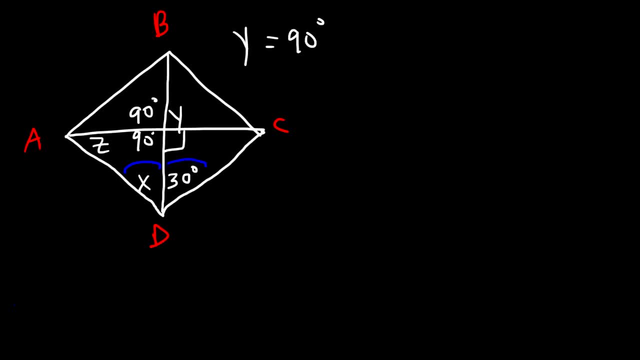 angle ADB has to be congruent to angle CDB. so if these two are equal to each other, that means X has to equal 30. now we can calculate Z. so if we focus on the this triangle, we can see that this is 90, this is Z and this is 30. so Z plus 30. 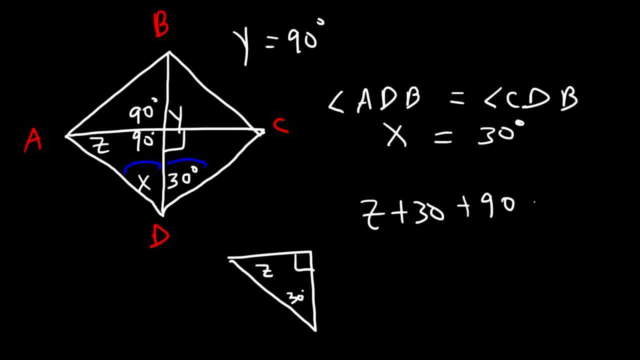 plus 90. the three interior angles of a triangle must add up to 180. 30 plus 90 is 120 and 180 minus 120 is 60. so these two angles, they're complementary to each other. they have to add up to 90 and these: 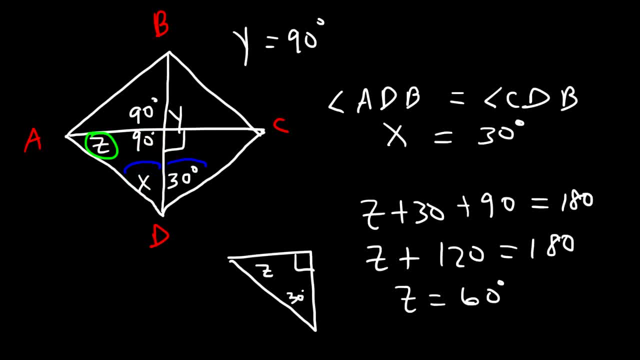 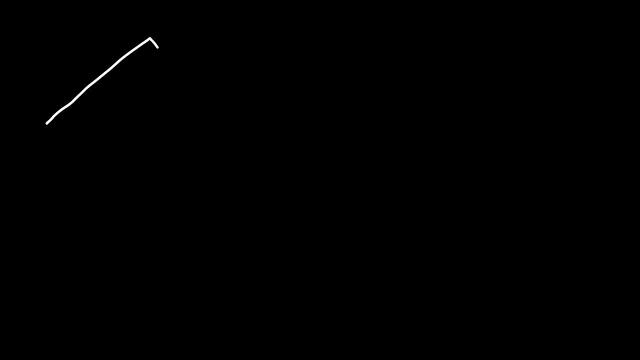 three in combined they have to add up to 180. so that's how you could calculate the missing angles of rhombus. so here's the next example problem that you can work on. so once again we have rhombus ABCD and this is going to be E. so let's say that. 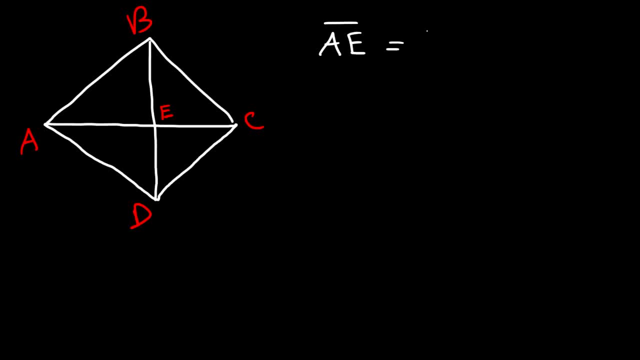 a, e is equal to three x plus a, 1x plus a plus 1.. And EC is equal to 5x minus 9.. So with this information, and let's say that also AB is 20. So with this information, calculate the value of DE. So go ahead and pause the. 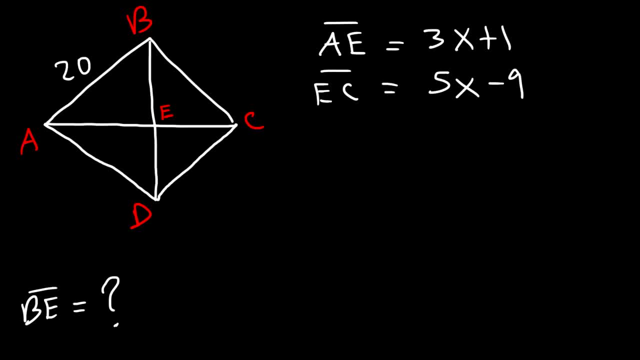 video. Try this problem. So we know that AE and EC are congruent because each diagonal bisects the other one. They're perpendicular bisectors of each other, which makes E the midpoint of AC. So therefore we could say that AE and EC are equal to each other, which 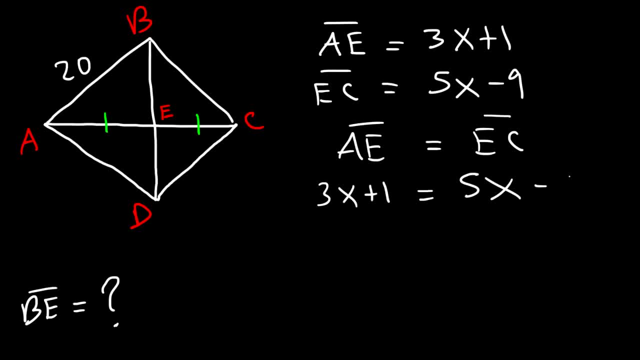 means that 3x plus 1 is equal to 5x minus 9.. So let's subtract both sides by 3x and let's add 9 to both sides, So 9 plus 1 is 10.. And 5x minus 3x is 2x. Now let's divide both sides by 2.. So 10 divided by 2 is 5.. So x. 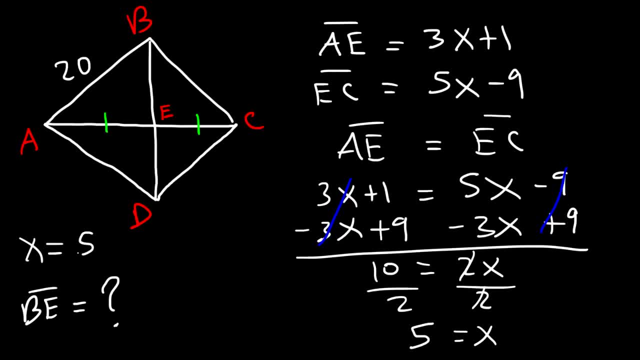 divided by 2 is 5, so X is equal to 5. so now that we have the value of X, we can calculate the measure of AE, which is 3x plus 1, so that's gonna be 3 times 5 plus 1. so 3 times 5 is 15 plus 1. 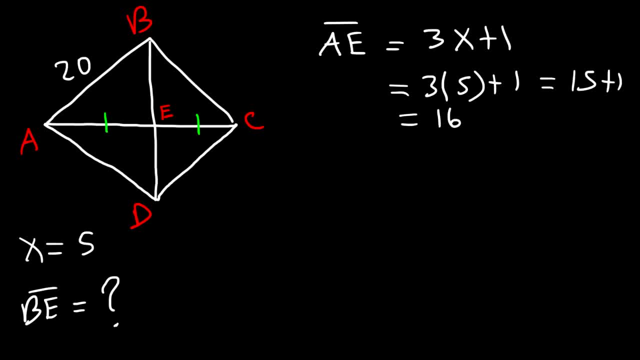 that's equal to 16. so AE is 16 and we know this is the right angle. so to calculate BE, which we'll call X, we could use the Pythagorean theorem. so 16 squared plus X squared has to equal the square of the hypotenuse, which is 20 squared. 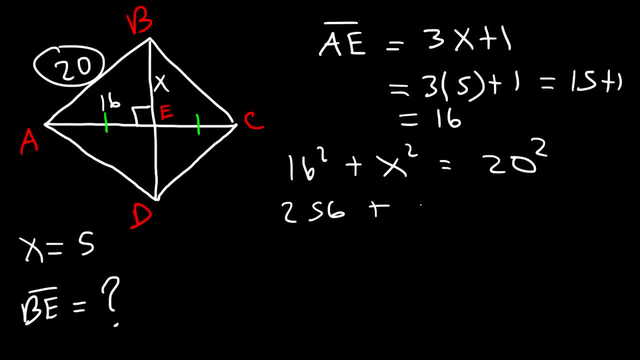 16 times 16 is 256, 20 times 20 is 400, and 400 minus 256 is 144. so if we take the square root of both sides, X is 12, which means that the measure of BE is 12 as well, and so that's how you can calculate it. now let's try a somewhat. 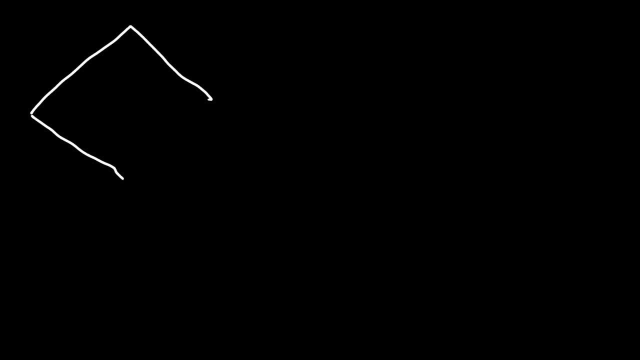 harder problem. so once again we have rhombus, ABCD and E is going to be the midpoint of the AC, just as before. so in this example, a? B is equal to y squared plus 1, and BC is equal to 3y plus 5, and also a? e that's going to be equal to 3x squared plus X. 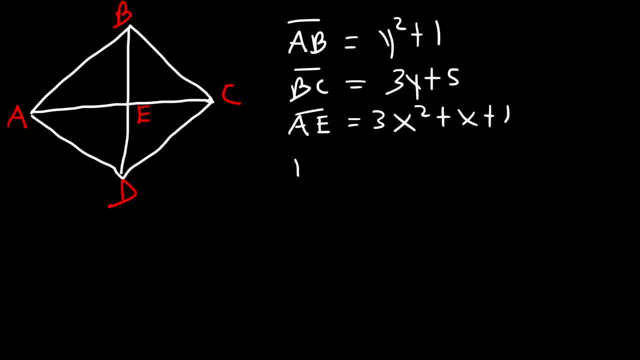 plus one and EC, that's going to be six x plus three. so with this information, your goal is to calculate the area of the rhombus. so feel free to pause the video and try. so the first thing that we can see is that all four sides of a rhombus are congruent. so therefore, A, B and BC are 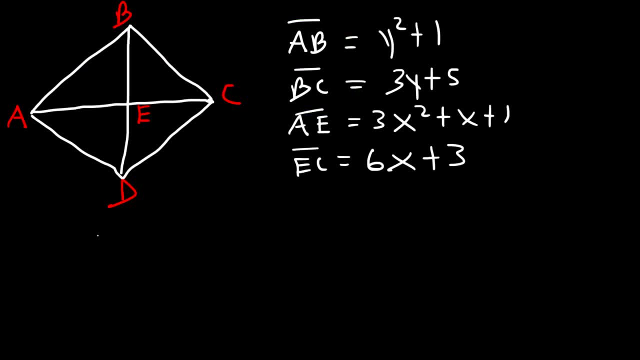 congruent to each other. so we could set y squared plus 1 equal to 3y plus 5.. So I'm going to take everything on the right side, move to the left. So y squared minus 3y plus 1 minus 5 is equal to 0.. So this: 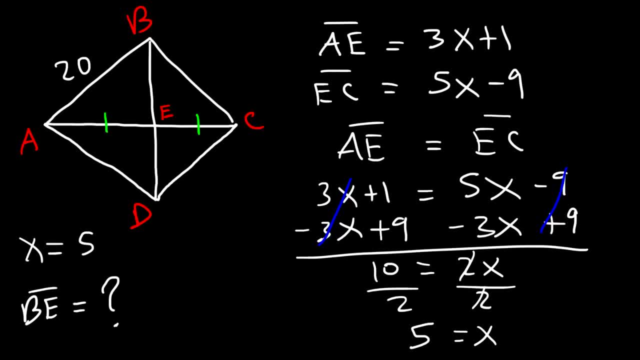 is equal to 5.. So now that we have the value of x, we can calculate the measure of AE, which is 3x plus 1. So that's going to be 3 times 5 plus 1. So 3 times 5 is 15 plus. 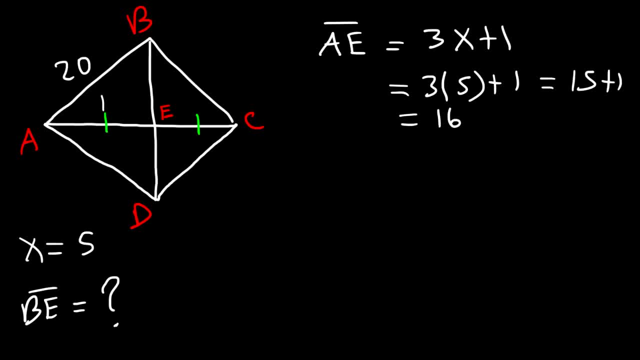 1. That's equal to 16. So AE is 16.. So AE is 16. And we know this is the right angle. So to calculate BE, which we'll call x, we could use the Pythagorean Theorem. So 16 squared plus x squared has to equal the. 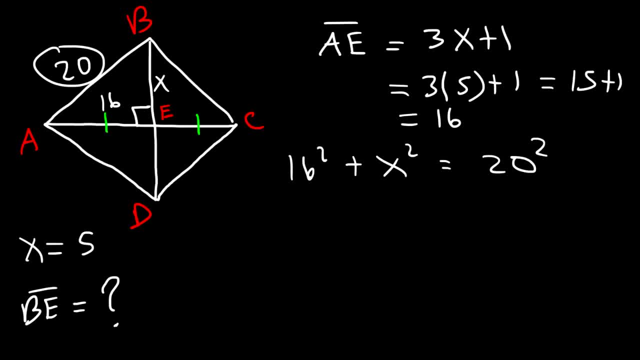 square of the hypotenuse, which is 20, squared 16 times 16 is 256.. 20 times 20 is 400.. And 400 minus 256 is 144.. So if we take the square root of both sides, x is 12, which we're going. 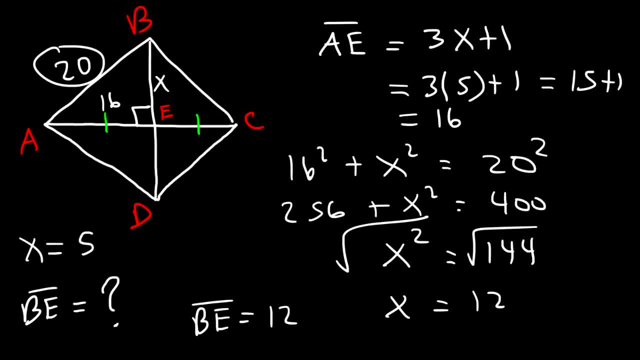 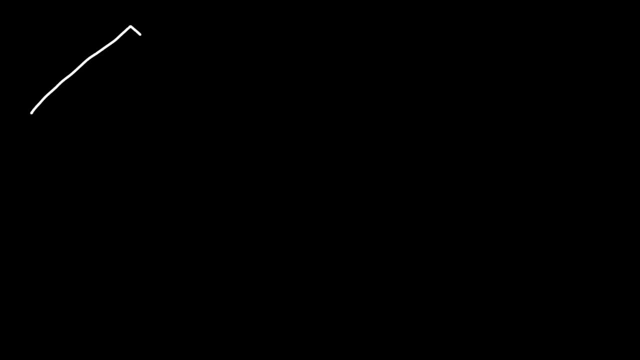 to calculate. we're going to get a margin, Ze, meaning that the measurement of BE is 12. well, And S. that's how you will calculate it now. So let's try a somewhat harder problem. So once again, we have Rhombus A. 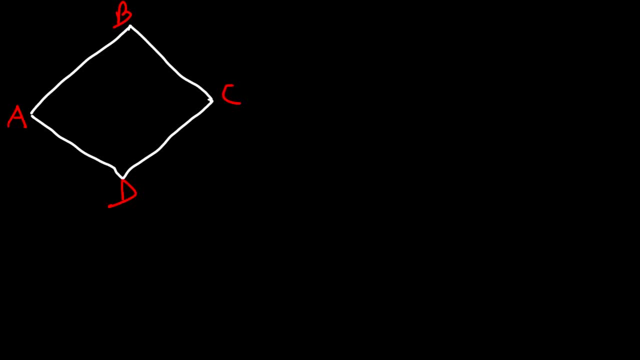 B, C, D, E will be the midpoint of AC, just as before. So in this equation we pictures, For example, AB is equal to y squared plus 1,, BC is equal to 3y plus 5, and AE is equal to 3x squared plus x plus 1, and EC is equal to 6x plus 3.. 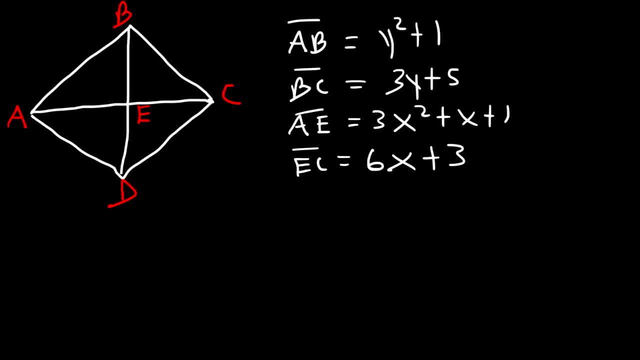 For this information. your goal is to calculate the area of the rhombus, So feel free to pause the video and try it. So the first thing that we can see is that all four sides of a rhombus are congruent. So therefore, AB and BC are congruent to each other. 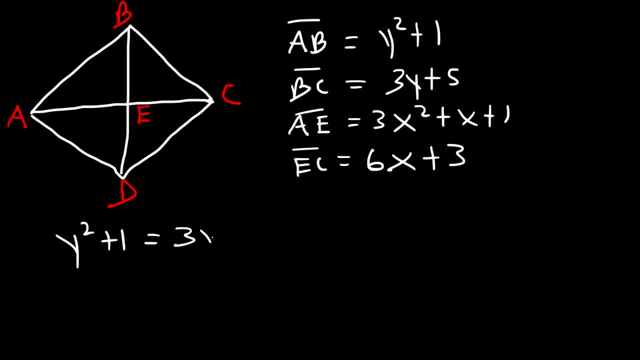 So we can set y squared plus 1 equal to 3y plus 5.. So I'm going to take everything on the right side and move it to the left. So y squared minus 3y plus 1 minus 5 is equal to 0.. 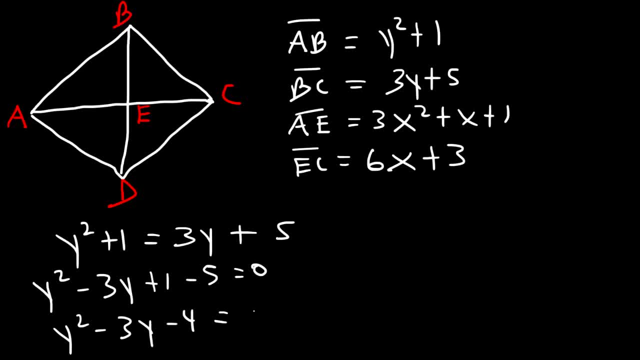 So this becomes y squared minus 3y minus 4.. Now, in order to factor this expression, we need two numbers that multiply to negative 4, but add to negative 3. And so this is going to be negative 4 and positive 1.. 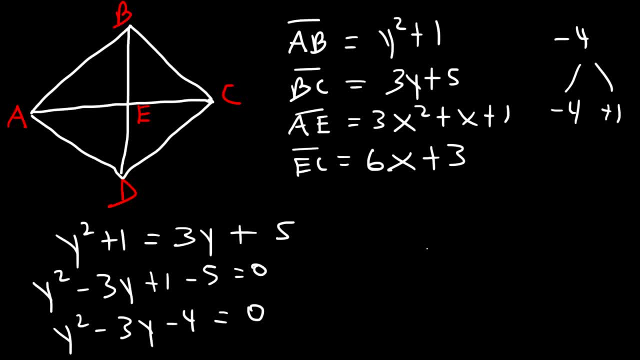 Negative 4 times 1 is negative 4, but negative 4 plus 1 adds up to negative 3.. So to factor it's going to be y minus 4.. Times y plus 1. Which means y can equal 4, or it could be negative 1.. 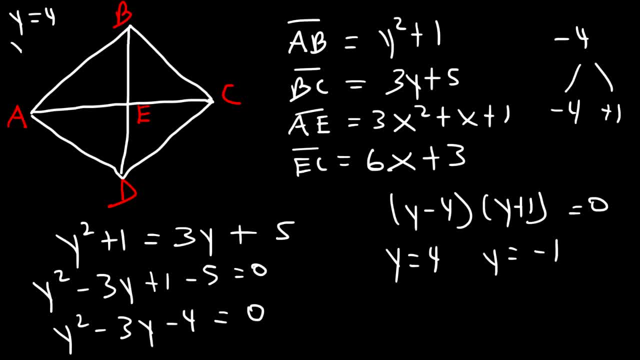 So let me write that on the side somewhere, Because both answers can work. So let's calculate AB when y is negative 1.. So it's y squared plus 1.. That's negative 1 squared plus 1., Which is 1 plus 1, so that's 2.. 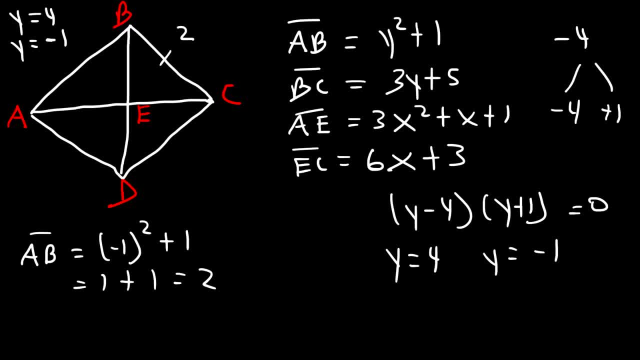 So that's one possible answer which I'm going to write over here. So AB and BC could be 2.. Now, if y is 4, we can get a different answer: 4 squared plus 1. 4 squared is 16.. 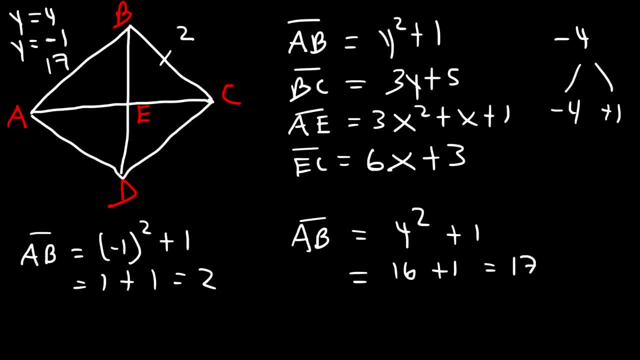 16 plus 1 is 17.. So AB could be 17.. So we have these two possible values, And so in time we'll see which is the best one to use. So now let's focus on AE and EC. E is the midpoint of AC. 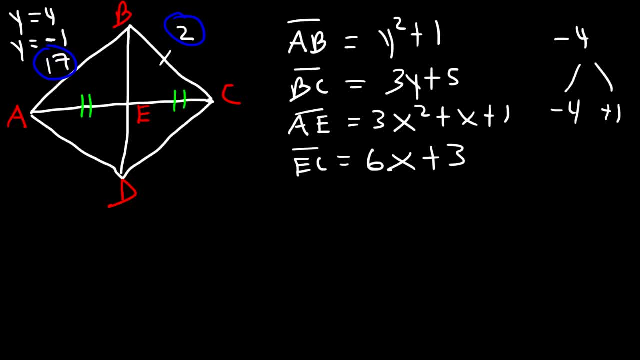 So AE and EC are congruent. So this time We can set 3x squared plus x plus 1, equal to 6x plus 3.. So let's move everything to the left side. So this is going to be x minus 6x, which is negative 5x. 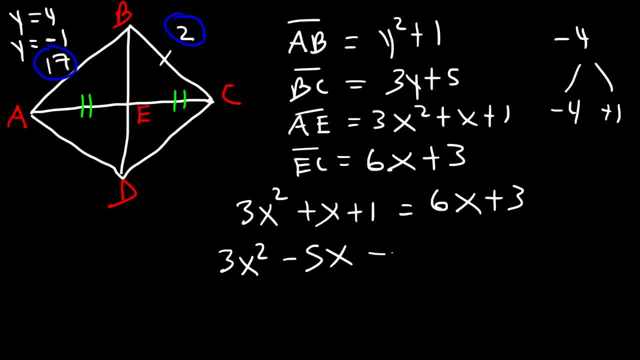 And then 1 minus 3.. That's going to be negative 2 on the left side. So how can we factor this expression? Because the coefficient is not 1 anymore. The leading coefficient is 3.. So how can we factor this expression? 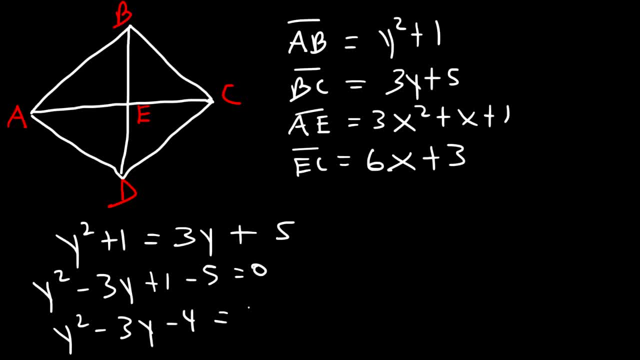 becomes y squared minus 3y minus 4.. Now, in order to factor this expression, we need two numbers that multiply to negative 4 but add to negative 3. And so this is going to be negative 4 and positive 1.. Negative 4 times 1 is negative. 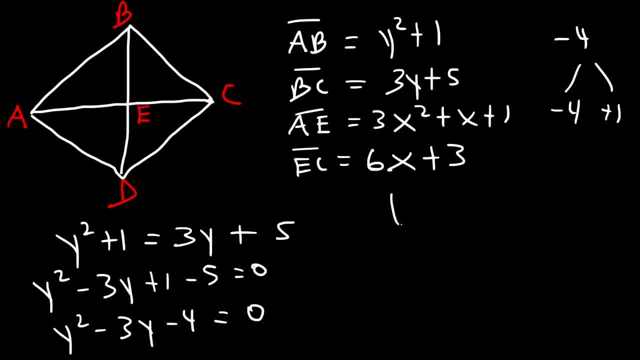 4, but negative 4 plus 1 adds up to negative 3. So to factor is going to be y minus 4 times y plus 1. Which means y can equal 4 or it could be negative 1.. So let me write that on the side somewhere. 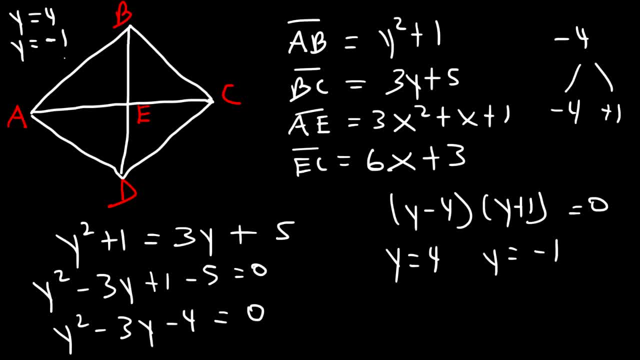 Because both answers can work. So let's calculate AB when Y is negative 1.. So it's Y squared plus 1, that's negative 1 squared plus 1, which is 1 plus 1, so that's 2.. 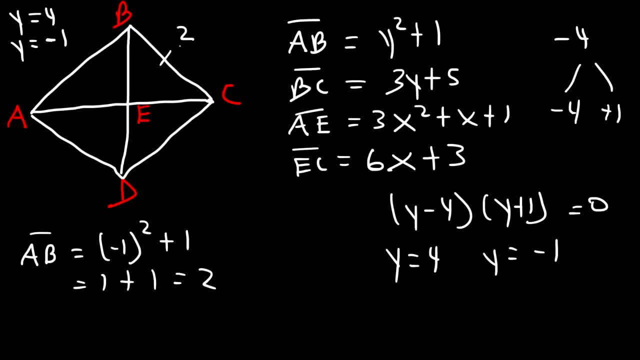 So that's one possible answer which I'm going to write over here. So AB and BC could be 2.. Now if Y is 4, we can get a different answer. So 4 squared plus 1.. 4 squared is 16, 16 plus 1 is 17.. 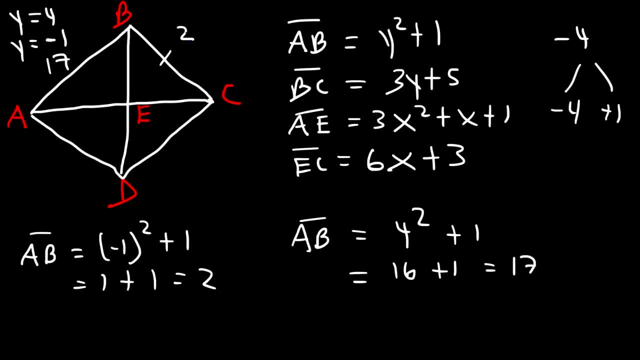 So AB could be 17.. So we have these two possible values, And so in time we'll see which is the best one to use. So now let's focus on AE and EC. E is the midpoint of AC, so AE and EC are congruent. 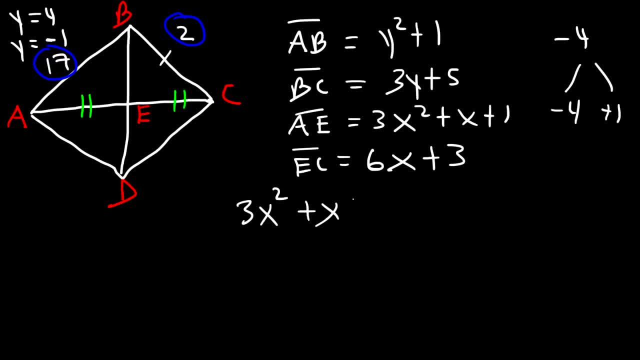 So this time we could set 3X squared plus X plus 1, equal to 6X plus 3.. So let's move everything to the left side. So this is going to be X minus 6X, which is negative 5X. 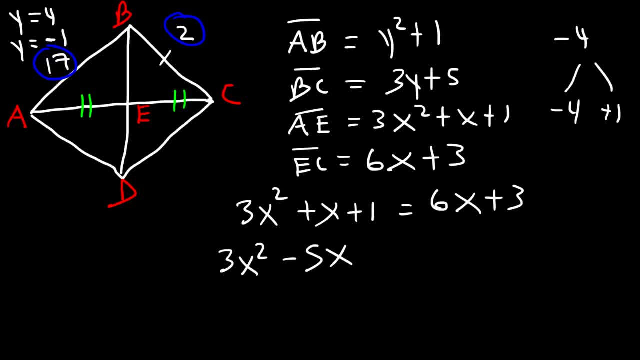 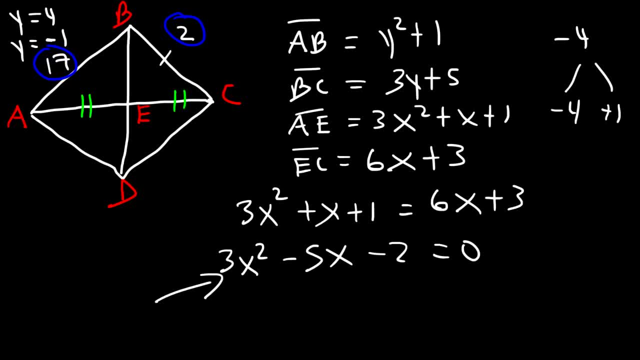 So how can we factor this expression? Because the coefficient is not 1 anymore. The leading coefficient is 3.. So what we need to do is multiply the leading coefficient by the constant term. 3 times negative, 2 is negative 6.. 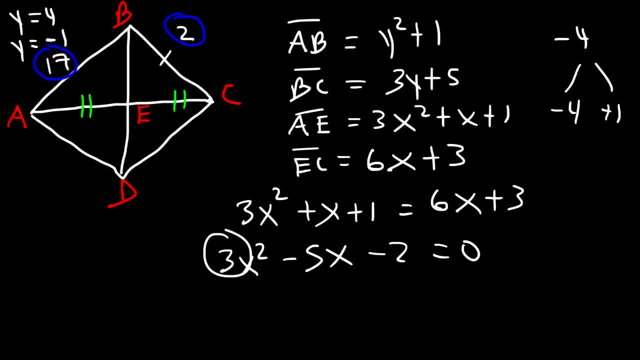 So what we need to do is multiply the leading coefficient by the constant term. 3 times negative 2 is negative 6.. And then find two numbers that multiply to negative 6 but add to negative 5.. So this is going to be negative 6 and 1.. 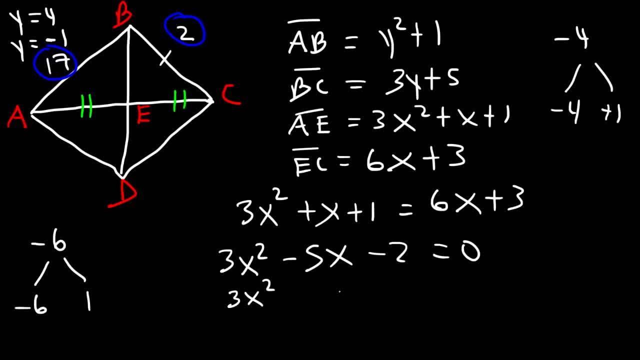 Negative 6 plus 1 is negative 5.. So now let's replace negative 5x with negative 6x plus 1x, And then we need to factor by grouping. So in the first two terms take out the GCF. 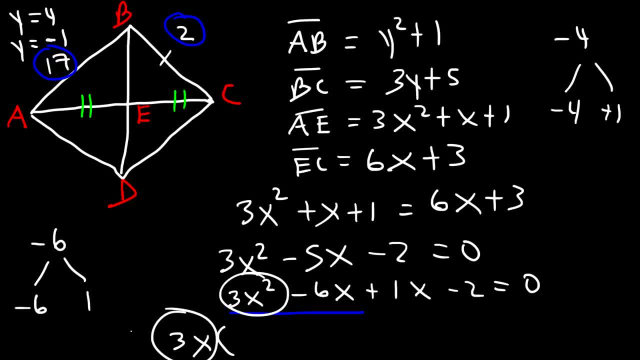 Which is 3x. 3x squared divided by 3x is x And negative. 6x divided by 3x is negative 2.. Now, in the last two terms, we can't take out anything except 1. This will give us the same factor, x minus 2, which is good. 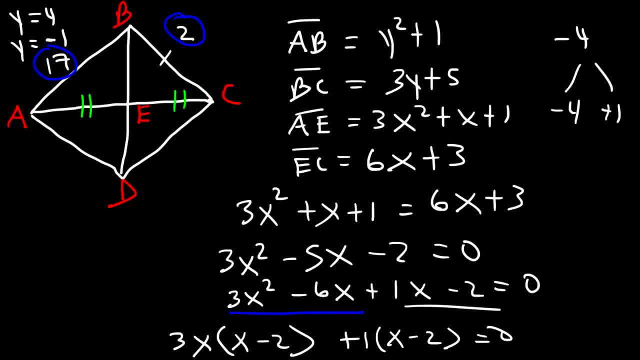 So now, if we take out x minus 2, we get negative 6x, And if we take out x minus 2, the stuff that will be inside the next parentheses is 3x plus 1.. So we have two possible answers. 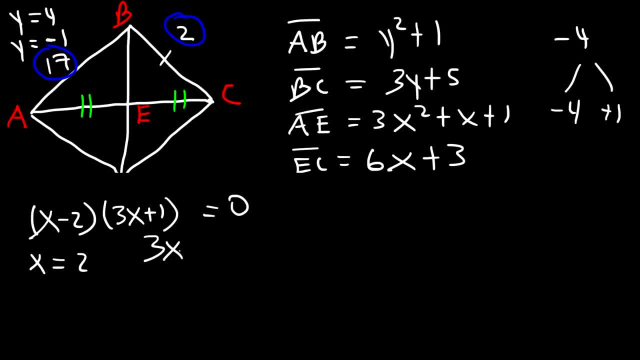 X is equal to 2, if we set that equal to 0. And if we set 3x plus 1 equal to 0. And if we subtract both sides by 1 and then divide by 3.. The second possible answer is: x is negative, 1 over 3.. 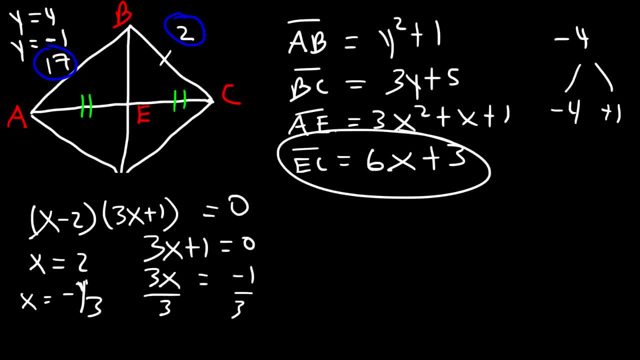 Okay. So let's use this expression. Let's plug in 2.. So if we plug in 2, this is going to be 6 times 2 plus 3.. 6 times 2 is 12.. 12 plus 3 is 15.. 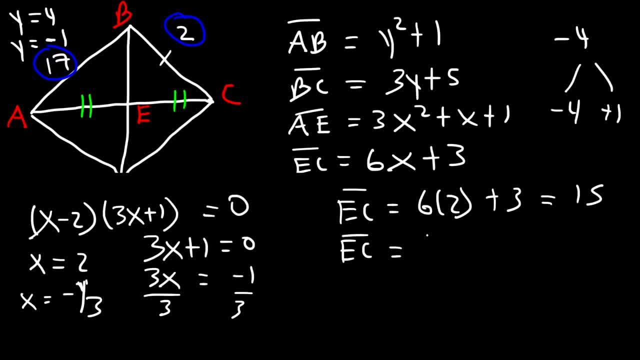 Now if we plug in, let's say, negative 1 third, it will be 6 times negative, 1 third plus 3.. So 6 divided by negative 3 is negative 2.. Negative 2 plus 3 is 1.. 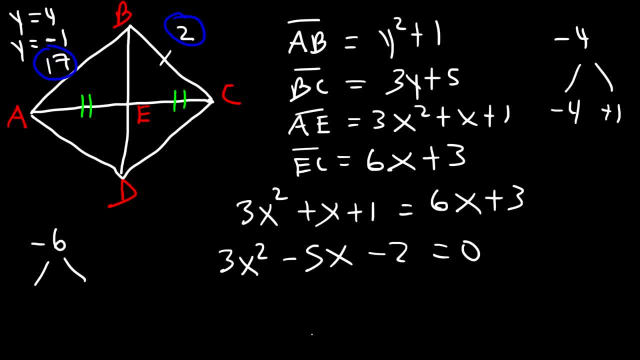 And then find two numbers that multiply to negative 6 but add to negative 5.. So this is going to be negative 6 and 1.. Negative 6 plus 1 is negative 5.. So now let's replace negative 5X with negative 6X plus 1X. 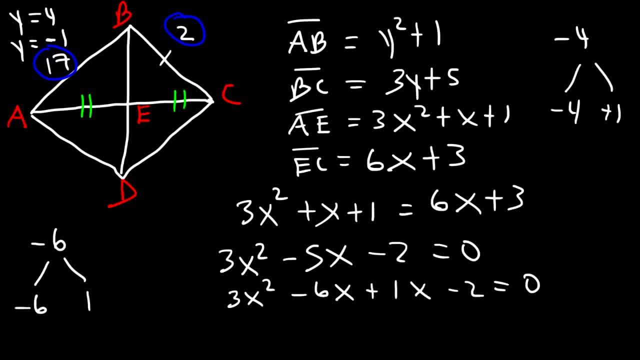 And then we need to factor by grouping. So in the first two terms, take out the GCF, which is 3X. 3X squared divided by 3X is X And negative. 6X divided by 3X is negative 2.. 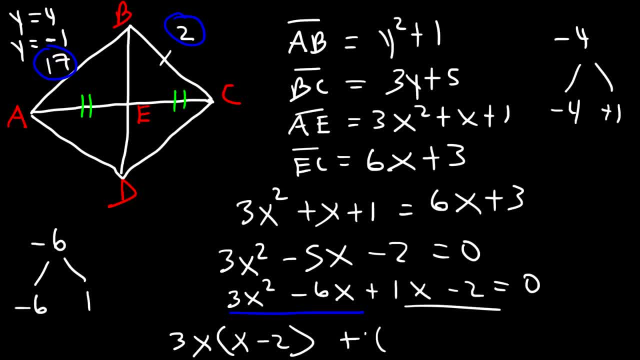 Now, in the last two terms, we can't take out anything except 1.. This will give us the same factor, X minus 2, which is good. So now, if we take out X minus 2, the stuff that will be inside the next parenthesis is 3X plus 1.. 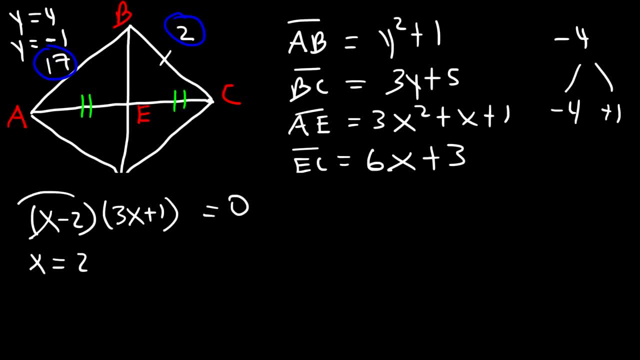 So we have two possible answers: X is equal to 2 if we set that equal to 0. And if we set 3X plus 1 equal to 0. And if we subtract both sides by 1. And then divide by 3.. 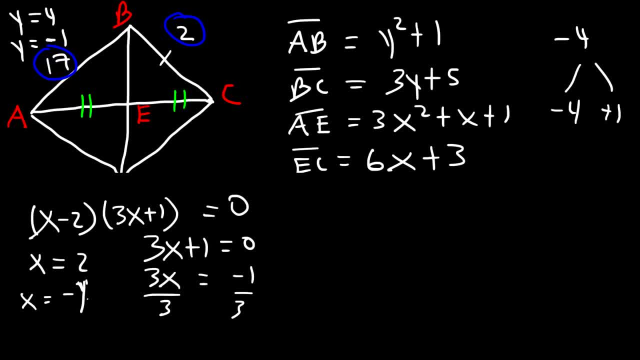 The second possible answer is: X is negative, 1 over 3.. So let's use this expression, Let's plug in 2.. So if we plug in 2, this is going to be 6 times 2 plus 3.. 6 times 2 is 12.. 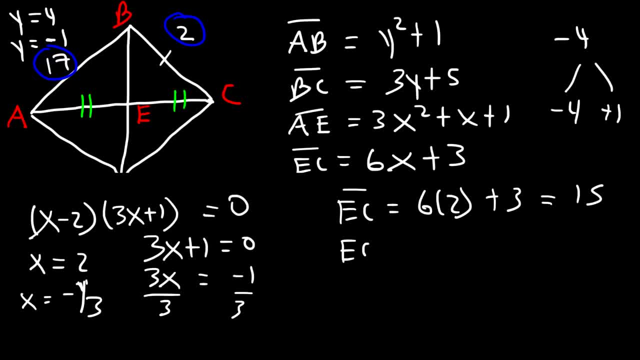 12 plus 3 is 15.. Now if we plug in, let's say, negative 1 third, It will be 6 times negative 1 third plus 3.. So 6.. 6 divided by negative 3 is negative 2.. 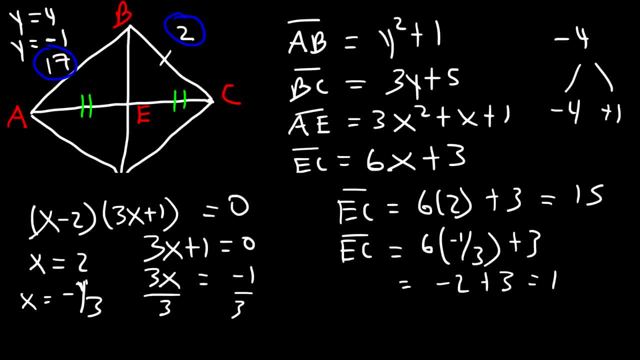 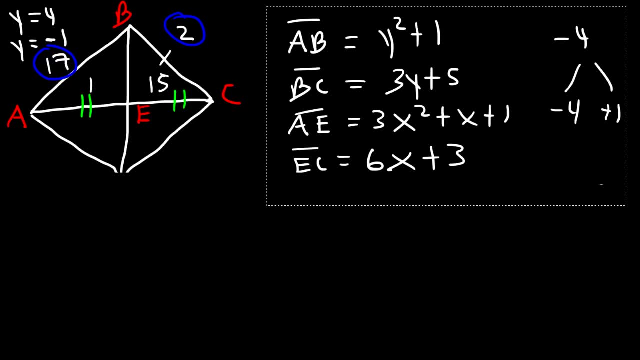 Negative, 2 plus 3 is 1.. So we have two possible answers: EC is either 15 or it could be 1.. So let's draw the possible figures that we could have. So if the hypotenuse is 17,, it's likely that AE and EC is 15.. 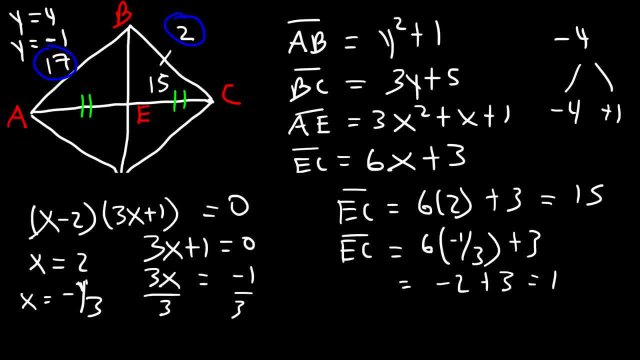 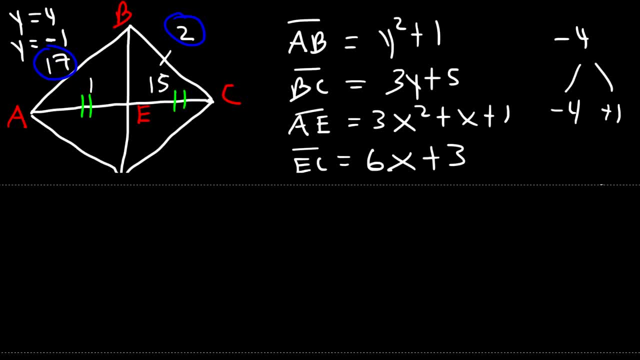 So we have two possible answers: E C is either 15 or it could be 1.. So let's draw the possible figures that we could have. So if the hypotenuse is 17,, it's likely that A E and E C is 15.. So if the hypotenuse is 17, it's likely that A, E and E C is 15.. So if the hypotenuse is 17,, it's likely that A, E and E C is 15.. Okay, 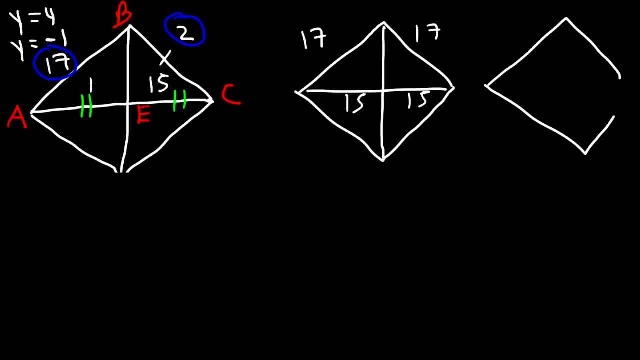 So if the hypotenuse is 17,, it's likely that A, E and E, C is 15.. And if the hypotenuse is 2, it's likely that this is 1 and this is 1.. Now let's find the missing side. 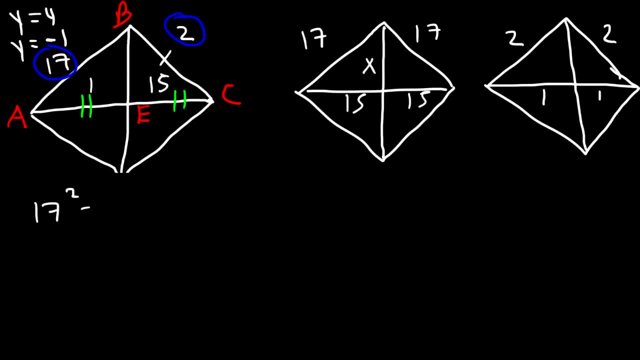 Let's call this X, So 17 squared has to equal X squared plus 15. squared 17 times 17 is 289.. 15 squared is 225.. And 289 minus 225 is 64.. Okay, And the square root of 64 is 8.. 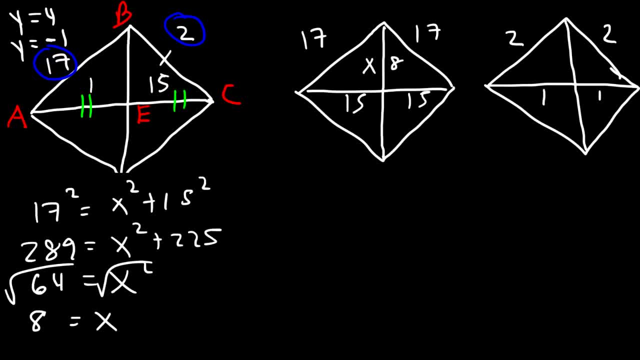 So that's a nice number. So this could be 8 and that could be 8.. Now for the other one we have: 2 squared is equal to 1 squared plus X squared. So this is 4, this is 1.. 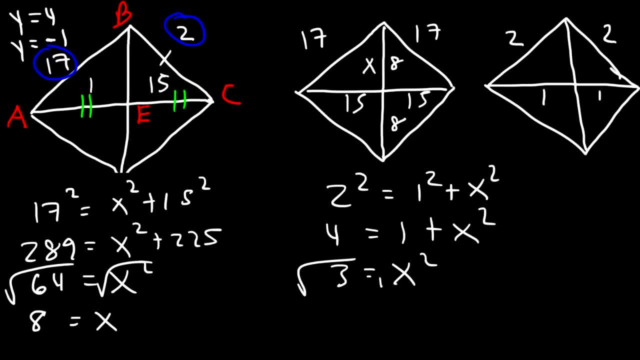 And so 4 minus 1 is 3.. Then, if we take the square root of both sides, this has to be the square root of 3.. So those are the two possible rhombus that we can get Now. granted, we can get another rhombus. 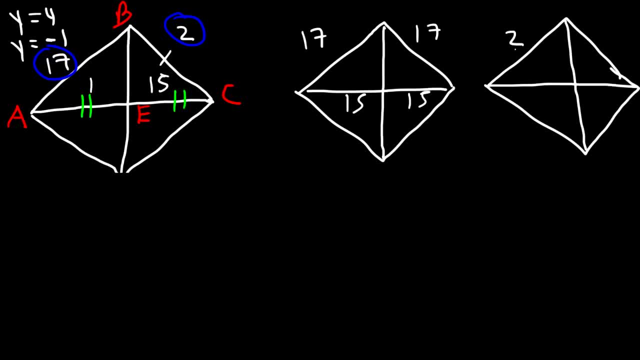 And if the hypotenuse is 2, it's likely that this is 1 and this is 1.. Now let's find the missing side. Let's call this X, So 17 squared has to equal X squared plus 15 squared. 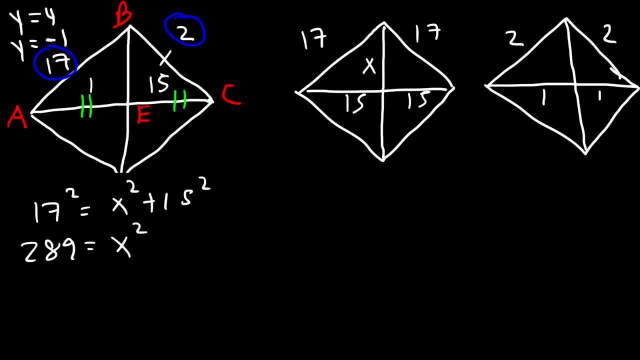 17 times 17 is 2A, 15 squared is 225.. And 289 minus 225 is 64.. And the square root of 64 is 8.. So that's a nice number. So this could be 8 and that could be 8.. 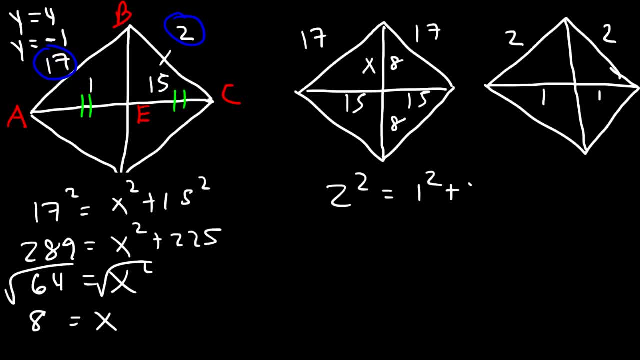 Now for the other one we have: 2 squared is equal to 1 squared plus X squared. So this is 4, this is 1., And so 4 minus 1 is 3.. Then if we take the square root of both sides, this has to be the square root of 3.. 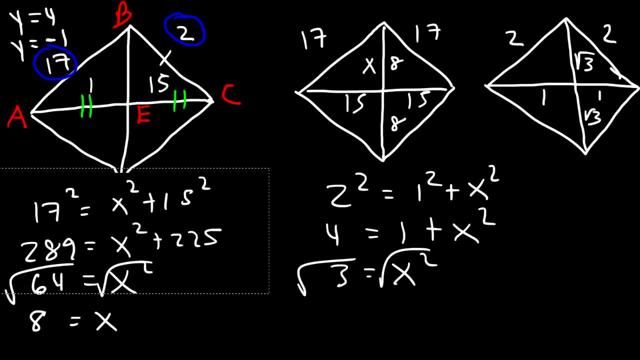 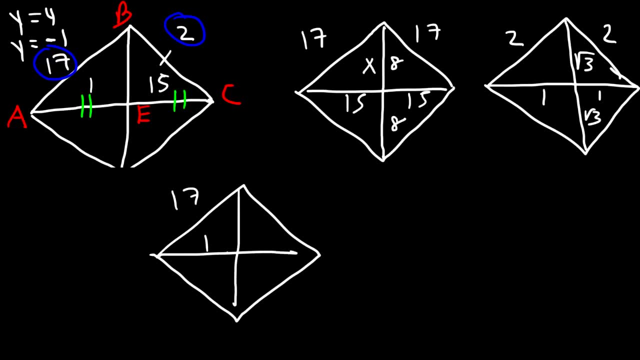 So those are the two possible rhombus that we can get Now. granted, we can get another rhombus where, let's say, if we chose a hypotenuse of 17 and this is 1.. So then 17 squared minus 1 squared would be like 288.. 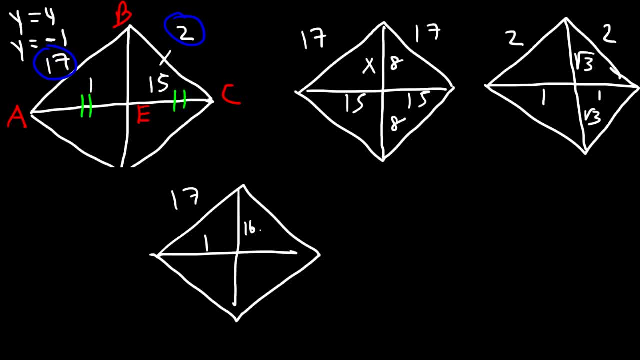 And the square root of that is basically 16.97.. This could happen, but I'm not going to worry about it. I'm going to worry about this one, And I'm not going to worry about this one too. Now, granted, you can calculate the area of that particular rhombus. 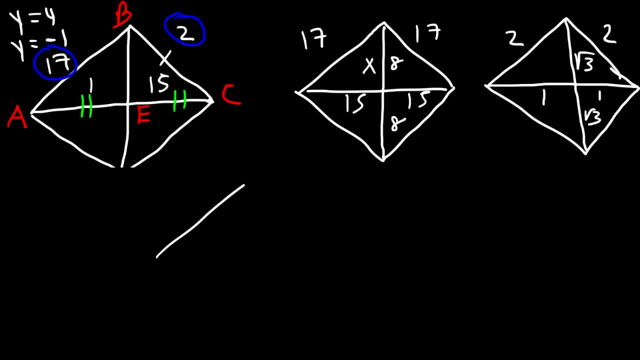 Where, let's say, if we chose a hypotenuse of 17 and this is 1.. So then 17 squared minus 1 squared will be like 288.. And the square root of that is basically 16.97.. This could happen, but I'm not going to worry about this one. 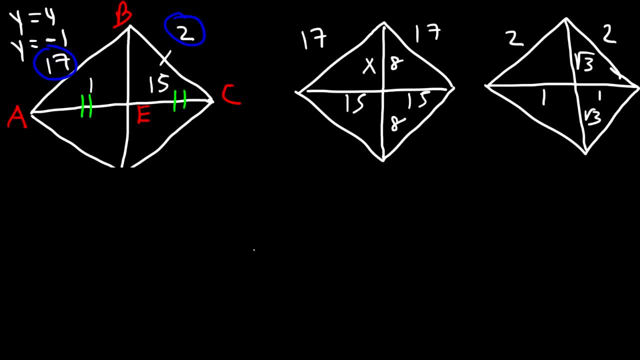 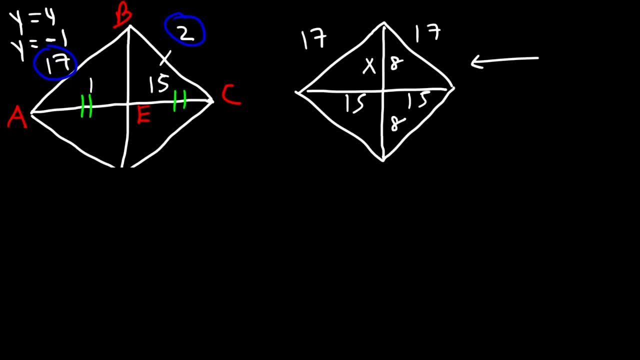 So I'm just going to focus on this example and you can repeat it for the other ones if you want to. Now the area is going to be 1 half D1 times D2.. So D1, we can see it's 8 plus 8, so that's 16.. 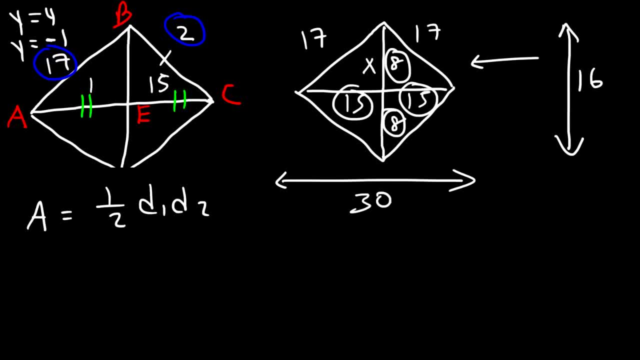 D2, it's 15 plus 15. Which is 30. So for this particular rhombus, the area is going to be 1 half 16 times 30. And half of 16 is 8.. 8 times 30 is 240.. 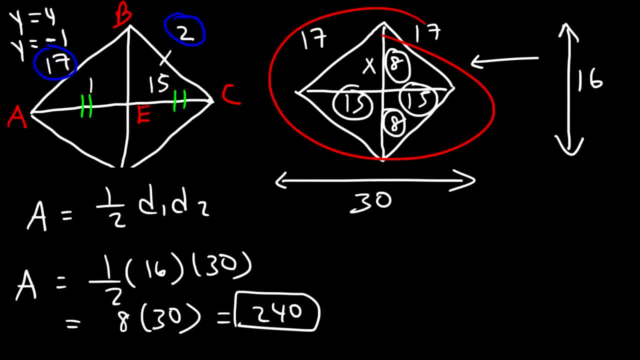 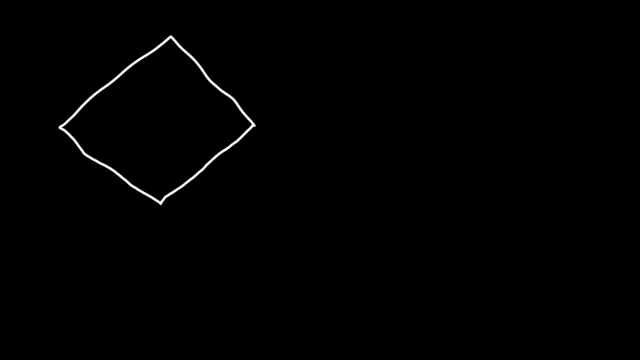 So this rhombus has an area of 240 square units. Now let's work on one more example. So let's say this is A, B, C and D, just like before, And in this example, let's say that A- C is equal to 3x. 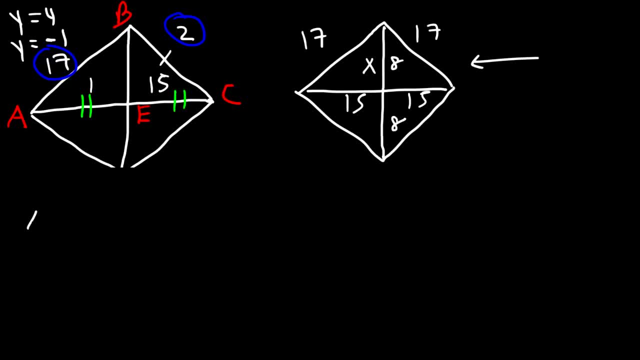 to focus on this example and you can repeat it for the other ones if you want to. Now the area is going to be 1 half D1 times D2.. So D1, we can see it's 8 plus 8, so that's 16.. 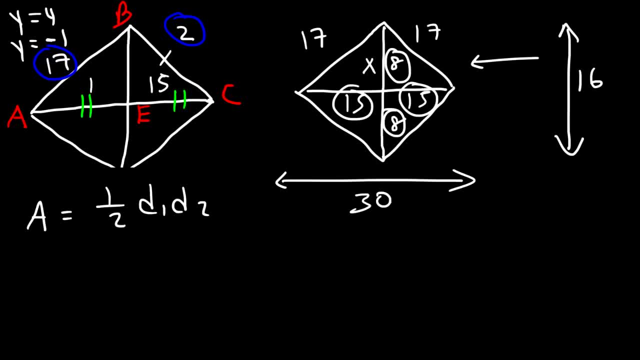 D2, it's 15 plus 15, which is 30. So for this particular rhombus, the area is going to be 1 half 16 times 30. And 1 half of 16 is 8,. 8 times 30 is 240.. 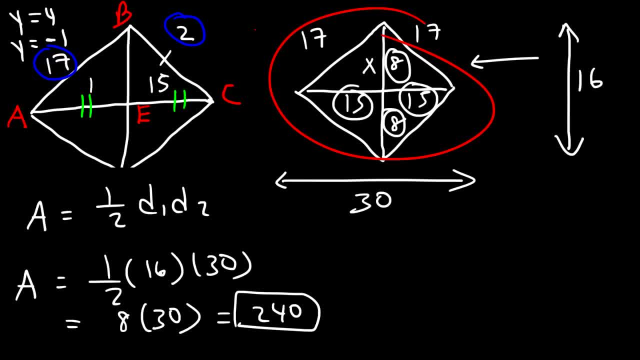 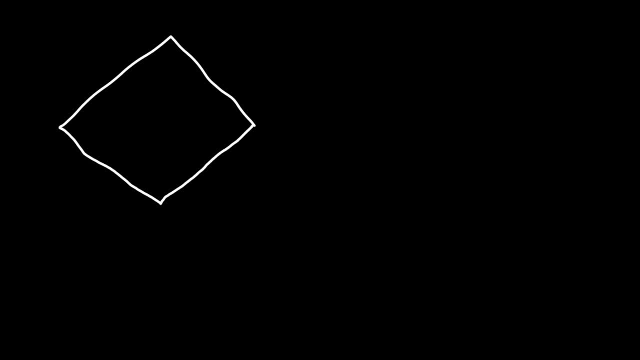 So this rhombus has an area of 240 square units. Now let's work on one more example. So let's say: this is A, B, C and D just like before. And this is A, B, C and D just like before. 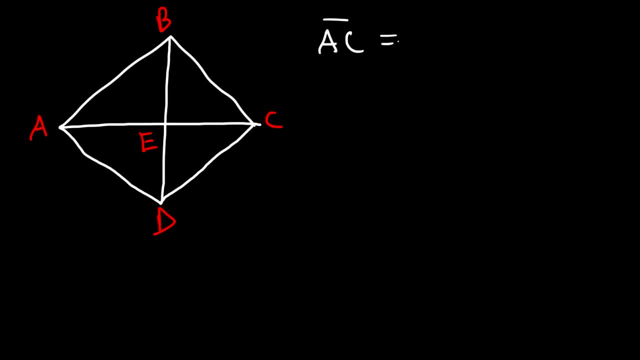 And in this example let's say that A C is equal to 3x and A E is x plus 4.. We're going to say angle B A D is 8y minus 2, and angle B A E is 4y minus 1.. 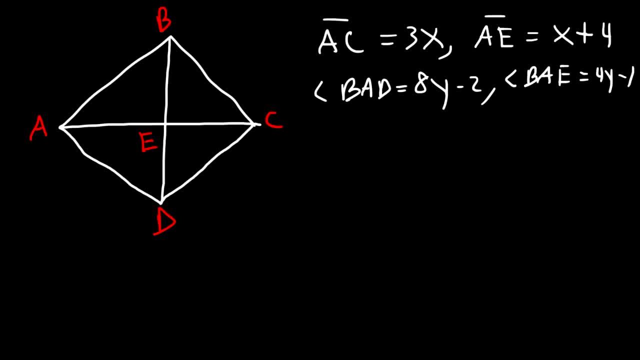 So, in this example, calculate the value of x and y. Now we know that A E and E C are congruent to each other. Now, what's the relationship between A C and A E? Well, let's say, if A E was 5, E C would be 5, but A C would be 10.. 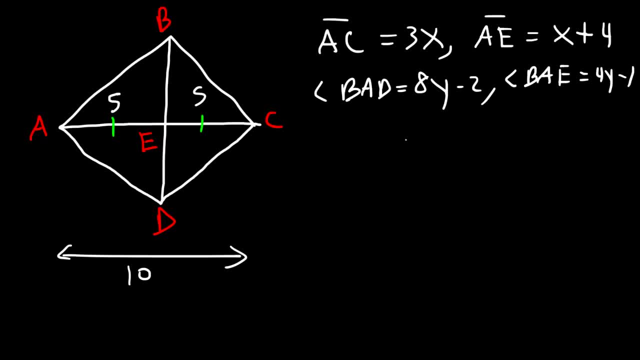 So the relationship between 5 and 10 is that 5 is half of 10.. So the 5 represents A E and the 10 represents A C. So A E is one half of A C. Now we have A E, it's x plus 4.. 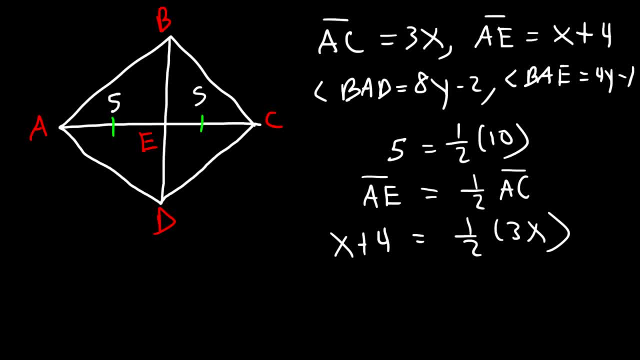 A, C is 3x, So now we can calculate the value of x. To get rid of the fraction, let's multiply both sides by 2.. So half times 2 is 1.. So we have 2x plus 8.. 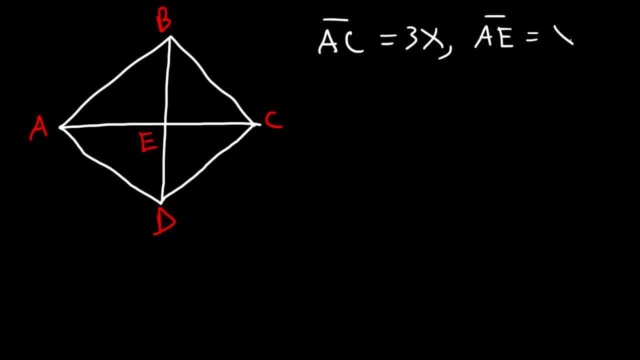 And A E is x plus 4.. We're going to say angle B A D is 8y minus 2.. And angle B A E is 4y minus 1. so in this example, calculate the value of x and y. now we 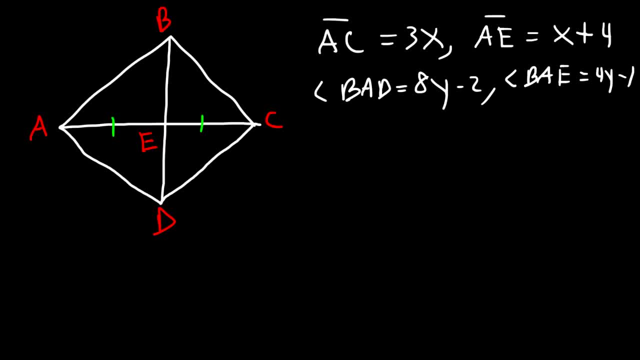 know that AE and EC are congruent to each other. now what's the relationship between a C and a E? well, let's say, if a E was 5, EC would be 5, but AC would be 10. so the relationship between 5 and 10 is that 5 is half of 10, so the 5 represents 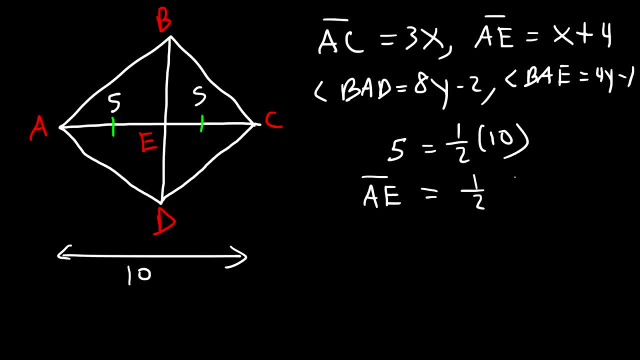 AE and a 10 represents AC. so a E is one half of a C. now we have AE, it's X plus 4. AC is 3x. so now we can calculate the value of X. to get rid of the fraction, let's multiply both sides by 2, so 1 half times 2 is 1. 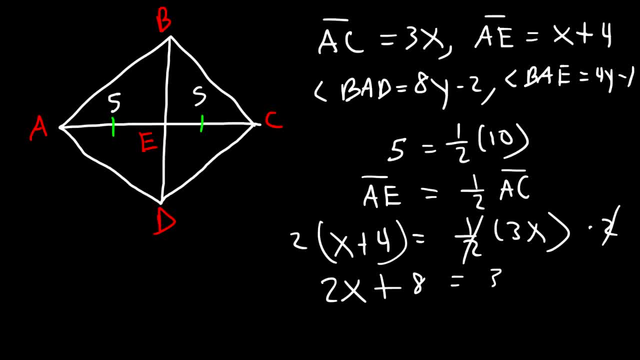 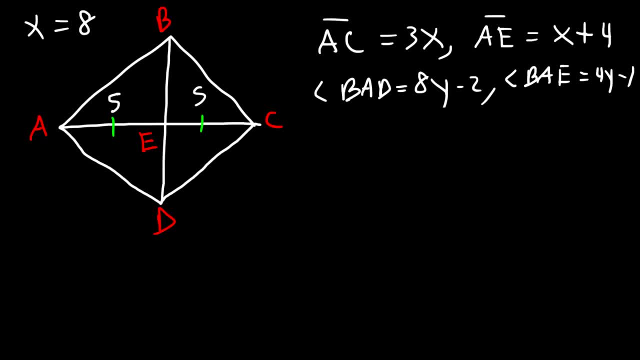 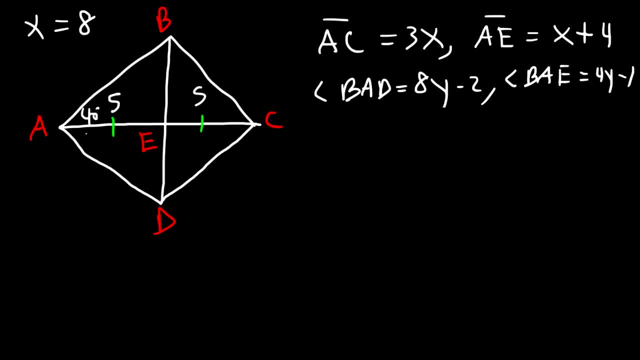 that means B ae would be 40 and dae would be 40. so 40 is half of 80. in this example the 40 would represent angle B ae, the 80 would represent angle B ad. so we could say that B ae is one half of B ad, so 4y.